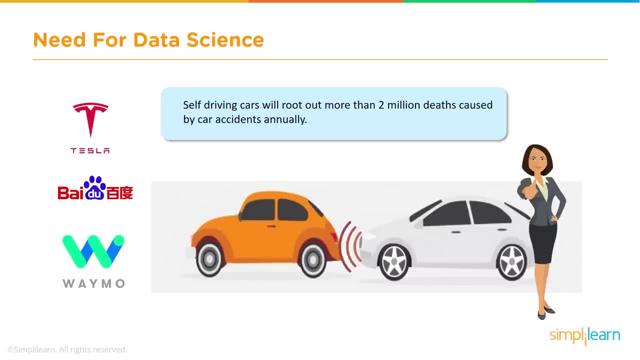 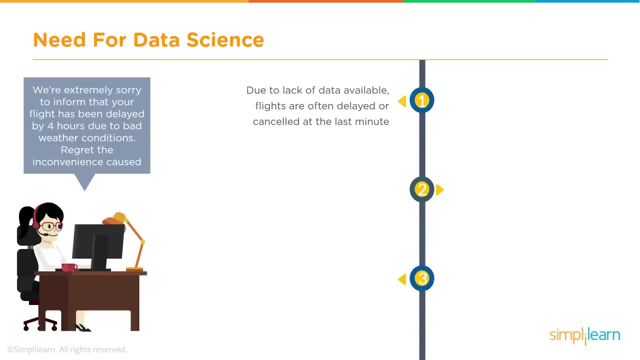 So we'll get started with our first question. Data science is investing in self-driving cars. So in about 10 to 15 years, some of the studies say that most of the cars will be autonomous or self-driving cars. Where else there are issues. for example, if we 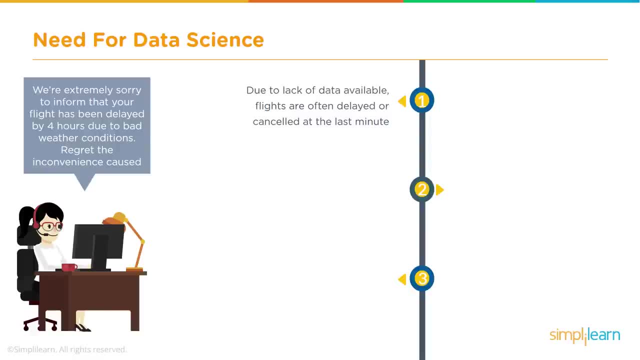 take airlines. this is another area where data science contributes in a major way. Flights get delayed due to weather conditions because the weather is not predicted in time, is not probably seen ahead of time. for all these unique data science, then this could be improper. 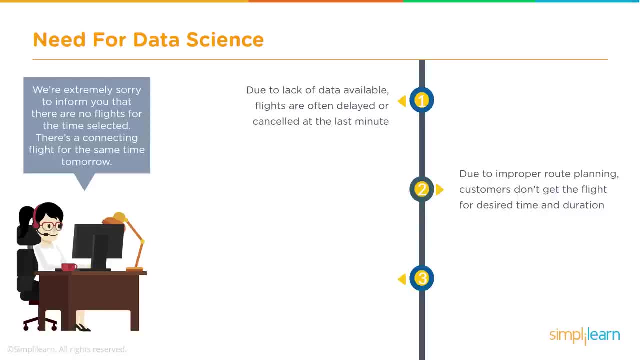 route planning and some customers might miss some flights. that again needs data science and similarly it could be incorrect decisions in selecting the right equipment, so which plane should fly in which route. that's the equipment that's being mentioned here. if that is not planned properly, then you might end up in a situation where the plane is not available whereas you 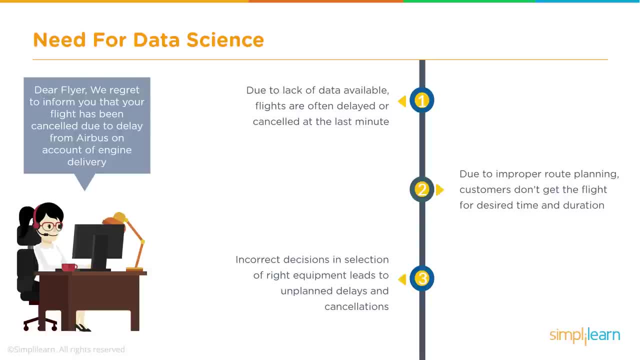 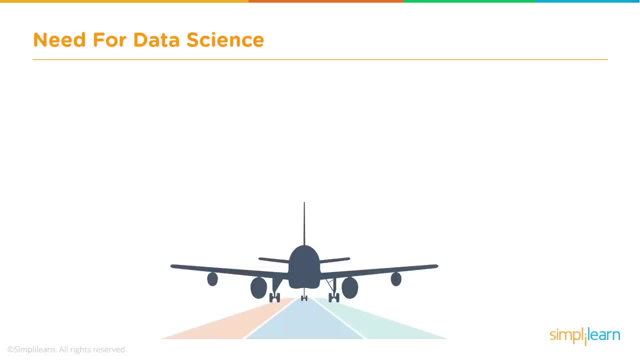 have planned for a flight in a particular route. so these are some of the challenges in one of the representative industries we are talking about, which is airlines. so, if we use data science properly, all of these or most of these problems can be avoided, and that will help in reducing. 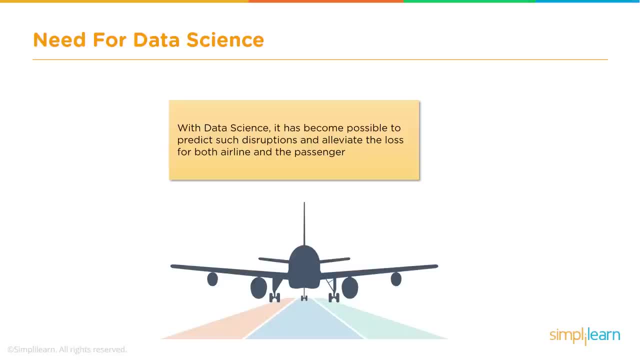 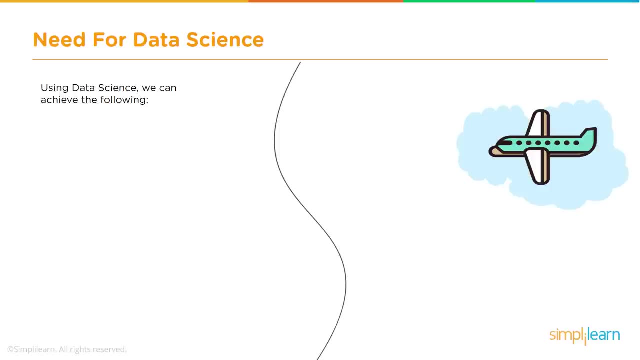 the pain both for the airlines and also for the passengers. a few more things that we need to know about data science. what else can we do? here are some of the other things that we can do, and we will stick to the airline industry. we can do better route planning so that there are less cancellations and less 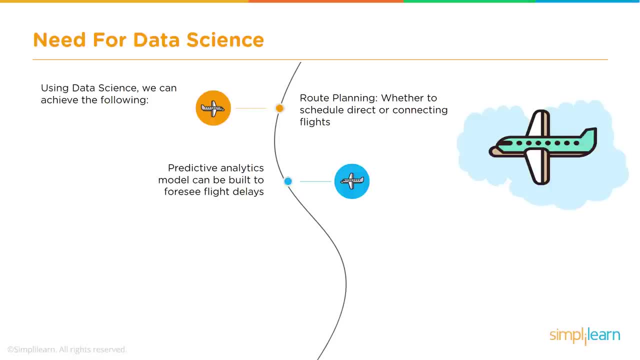 frustrated people. we can predict, use predictive analytics and predict any delays that are there, so that some flights can be rescheduled ahead of time. there are no last-minute changes. data science can also be used to make promotional offers. and the last but not least is what kind of planes should be used, or the different classes. 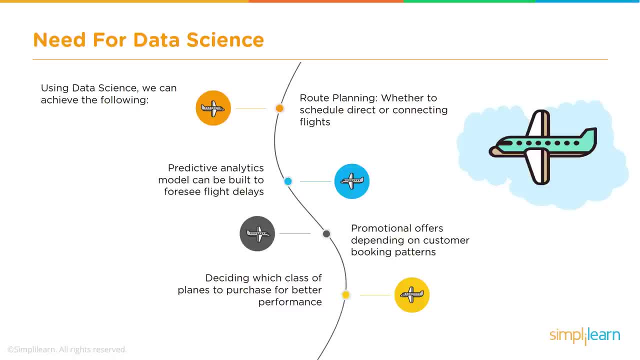 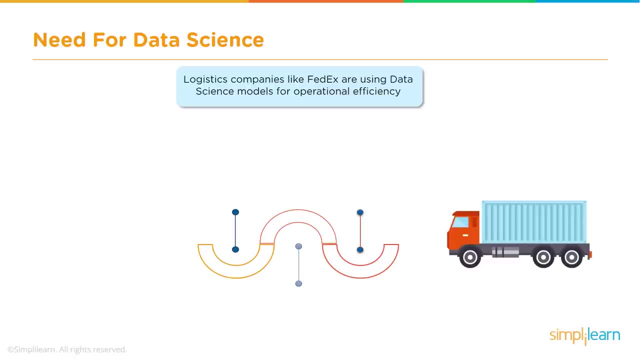 of planes that should be used in different routes for better performance. so these are some examples of how data science can be used in airlines, and another example or another industry where data science can be used and benefited would be in logistics. so companies like fedex, they use data. 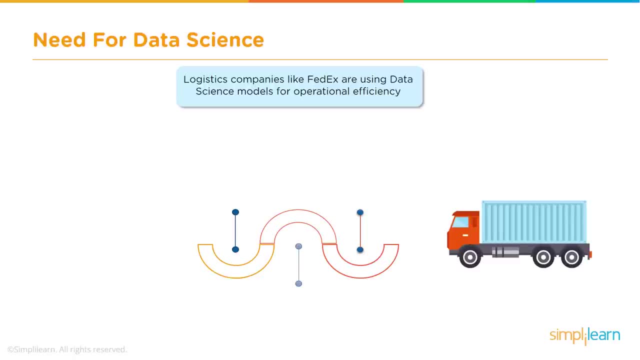 science models to increase their efficiency drastically, to optimize the routes and cut costs, and so on. so, before their delivery truck actually sets out, they determine which is the best possible route to ship their items to the customers and, based on various inputs, they also predict or come up with the best suited time to deliver. and, last but not least, they 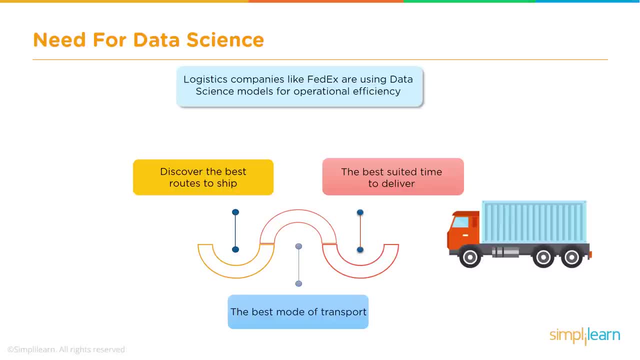 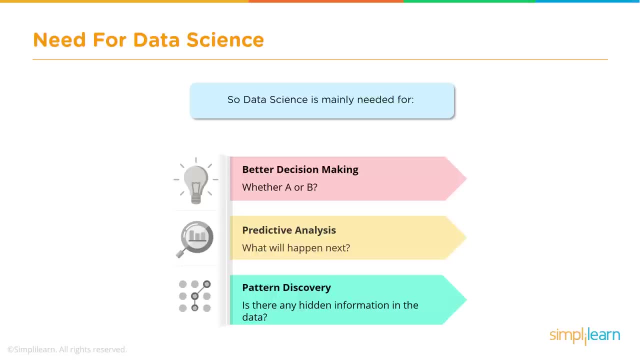 determine what is the best mode of transport for this delivery as well. so what is data science used for? these are some of the main areas where data science is used for better decision making. there are always tricky decisions to be made. so which is the right decision, which way to go so that 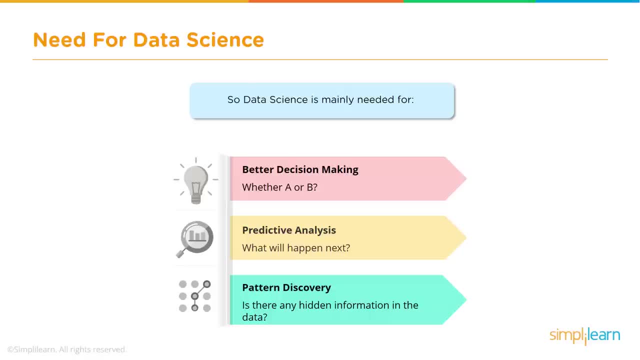 is one area, then, for predicting, for performing predictive analysis like, for example, can we predict delays, like in the case of airlines? can we predict the demand for certain products, let's say in e-commerce? that is the second area. the third area is pattern discovery or pattern creation. is there a pattern in which people are buying items? for example, it could be seasonality. 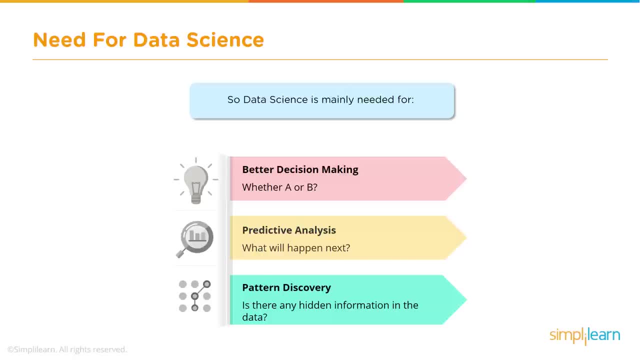 if you take the data, sales data for multiple years, there may be a pattern. in a way people are buying. that that's a buying pattern. certain months, probably, the sales will increase. certain months, the sales will come down certain quarters. traditionally, the sales will be higher certain quarters. so that is a pattern and this pattern discovery is another area where data science is. 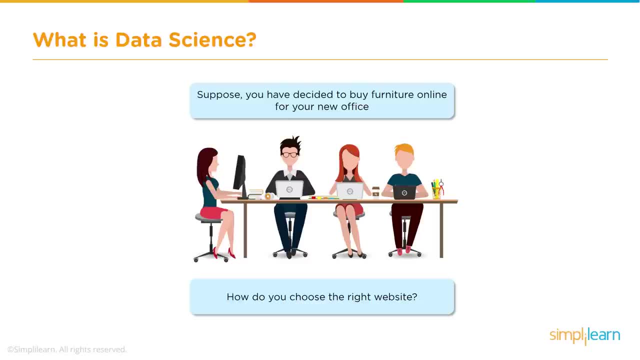 applied. what is data science now? let's take an example, a real life example. on a day-to-day basis, we use, or we try to make, some decisions. let's say, we want to buy some furniture online for our new office. so how do you go about doing this? you need to take a bunch of decisions to actually 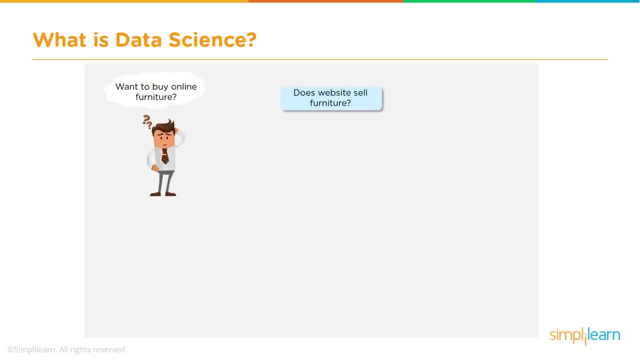 do the purchase. so we start with which website, which portal or which website you should use. so we try to find out. let's say you want to buy the furniture. obviously you don't go to a online grocery store because you need furniture, because there are several websites. so that is the. 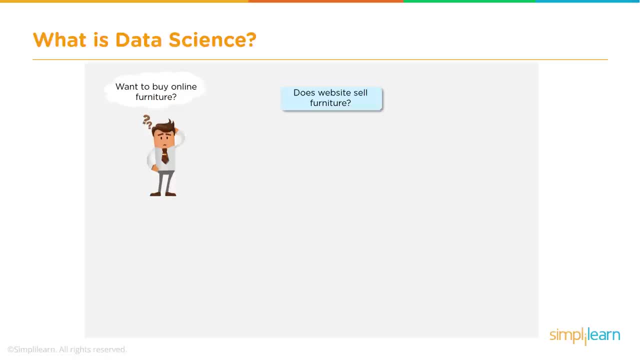 first decision you need to take which website i should use. so once we have multiple websites, you kind of discard all the websites which don't sell furniture and you stick to those websites which sell furniture. now, within that, we try to find out what is the ratings of this websites, if the 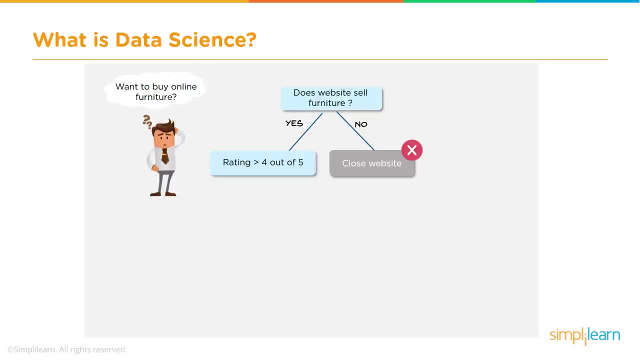 ratings is more, that means they are reliable, quality probably is good, and so on and so forth. so only then you want to buy from that particular website. so anything that doesn't satisfy this criteria, you close. all those websites. close in the sense you close the browser right, so you still are left with maybe a few of these which satisfy. 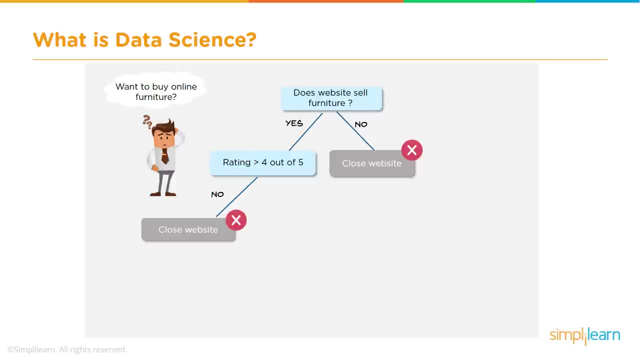 your criteria, that is, which sell web pages or websites that sell furniture. they have a rating of four and above. and then you look for discount. is somebody providing discount greater than 20 percent? then again you filter out some of them which probably are not providing any discount. 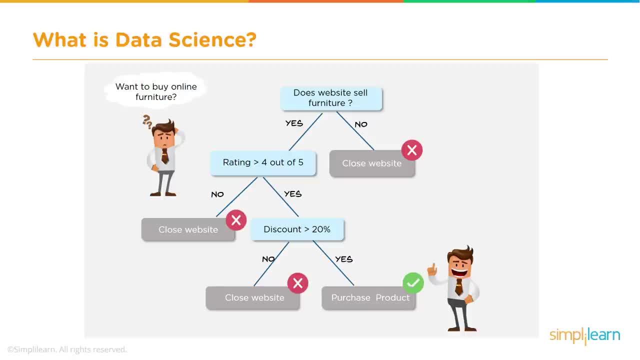 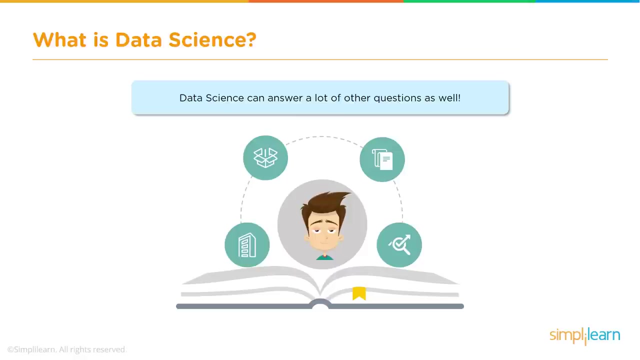 and zero down to one or two websites which are probably providing those discounts and go ahead and select the furniture and purchase it. so this is a very basic example. you probably don't follow this always exactly the same way, but just to illustrate, drive home the point so we can. 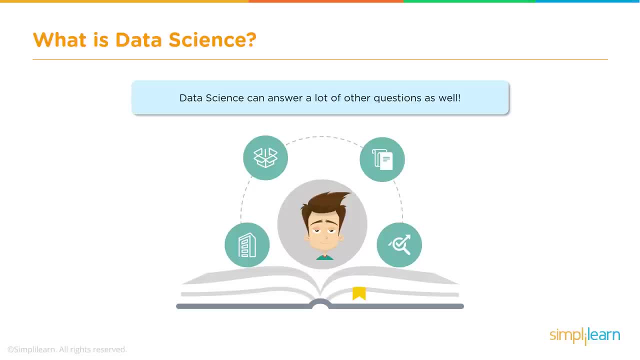 a lot of questions using data science. for example, when we take a cab, when we book a cab now to go from location a to location b, what is the best route that the cab can take to reach in the fastest way or in the least amount of time? there could be several factors. there could be traffic there. 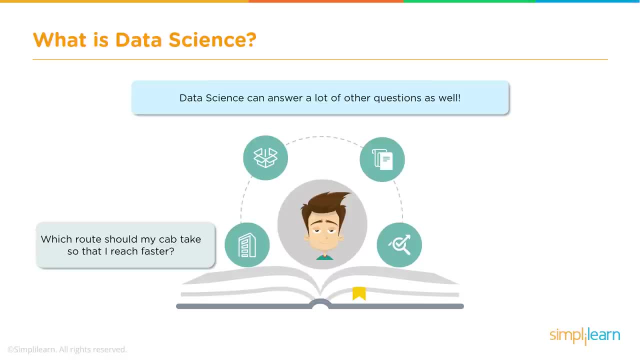 could be bad road, there could be weather. now all these come as inputs and a decision needs to be be taken as to which is the best route. Another example is TV shows, So Netflix and maybe even other, a lot of other TV channels. they have to perform this analysis to find out what kind of 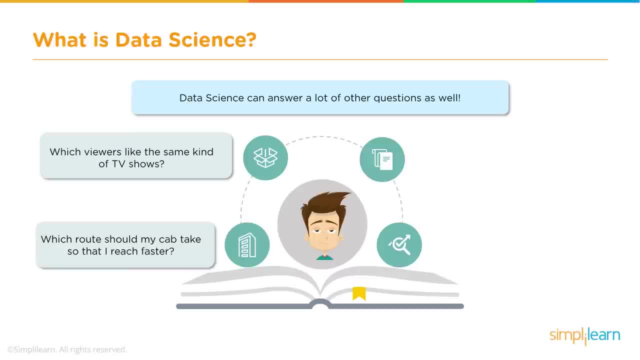 shows people are viewing, what kind of shows people are liking, and so on and so forth, so that they can then sell this information to advertisers, because their main source of revenue is advertising. So this is again a major function of data science: Predictive maintenance. We need to find out. will my 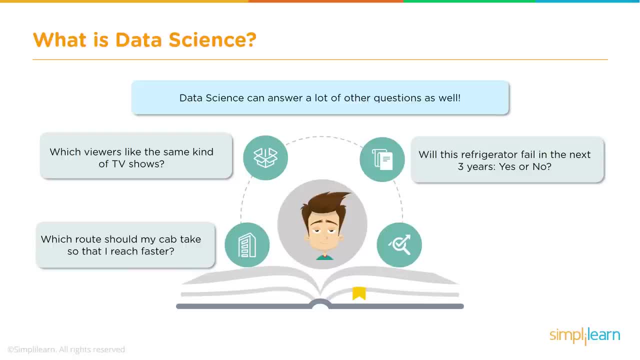 car break down? will my refrigerator break down in the next year or two years? should I be prepared to buy a new refrigerator? You can potentially apply data science here as well, And then in politics. a lot of data science is applied in politics. You must have seen on TV about US. 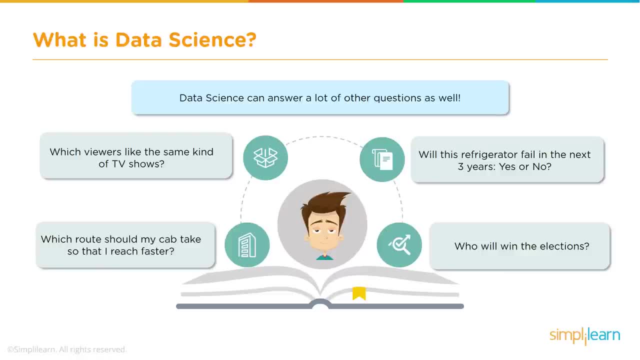 elections, or in UK or even in the United States. So this is a major function of data science. In India nowadays, everybody is applying data science in elections and trying to capture the votes, or rather, the voters, influence the voters. personalized messages: providing personalized 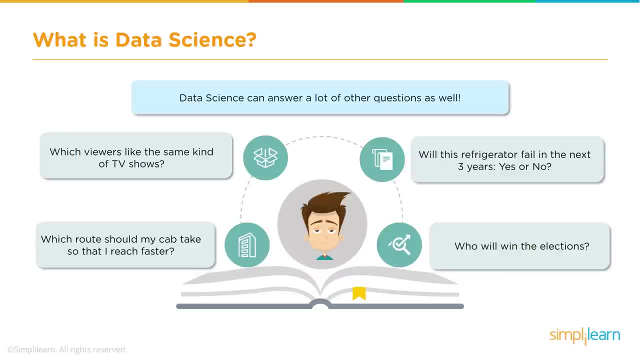 messages and so on and so forth, And that is one Not only that people use data science to even predict who is going to win the elections. It's a different matter that probably not all predictions come out to be true, But then 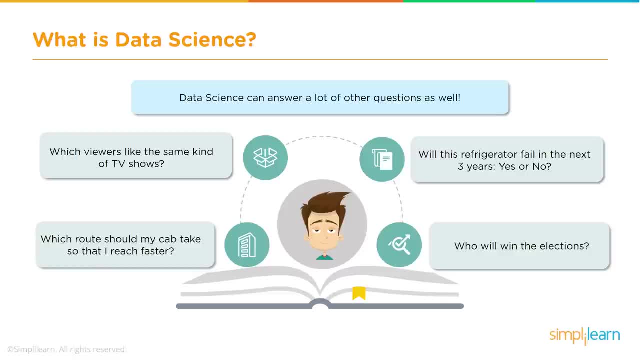 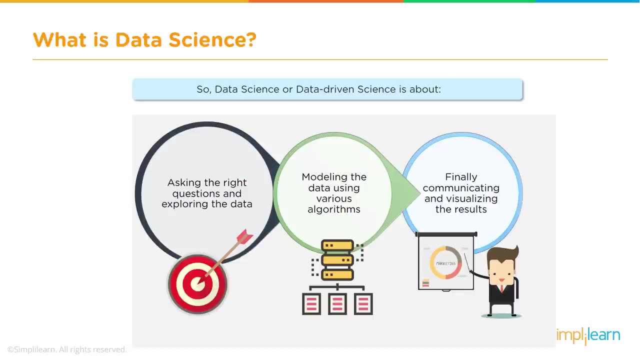 yes, this is. they use data science to do these predictions. So what is the process or what are the various steps in data science? The first step is asking the right question and exploring the data. Basically, you want to know what exactly is. 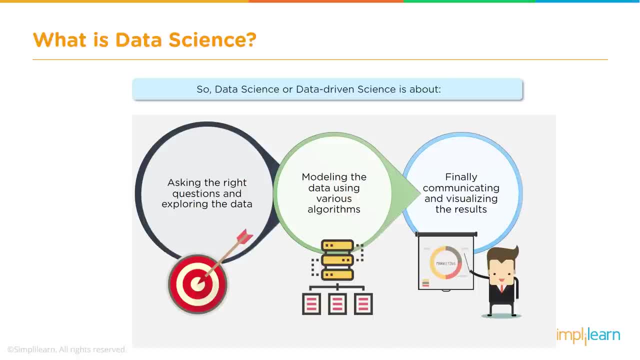 the problem you're trying to solve. So that is asking the right question. So that is the this circle out here. Then the next step is after exploring the data. So as a first step, you will ask some questions: What exactly is the problem you're trying to solve? 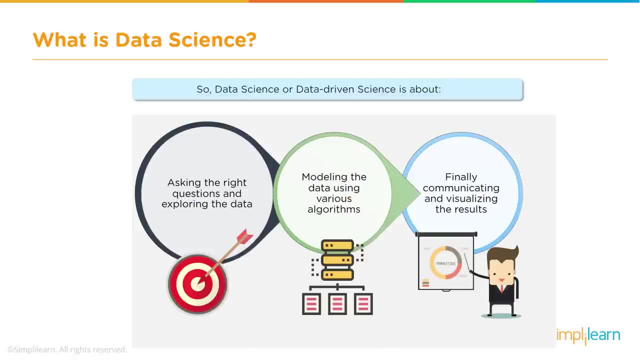 And then obviously you will have some data for that as input and you perform some exploratory analysis on the data. For example, you need to clean the data to make sure everything is fine, and so on and so forth. So all that is a part of exploratory analysis, And then you need to do: 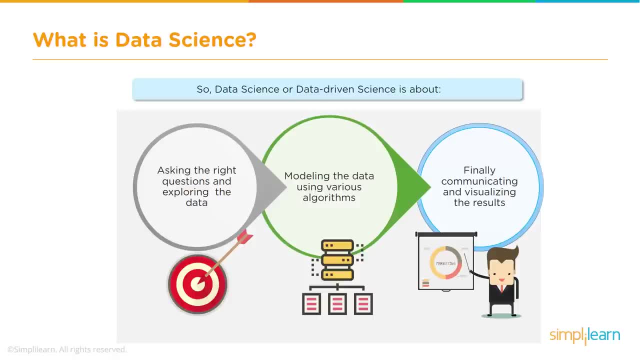 the modeling. Let's say, if you have to perform machine learning, you need to decide which algorithm to use and which model to use, And then you need to train the model, and so on and so forth. So that's all part of the modeling process, And then you run your data through this model and then through this process. 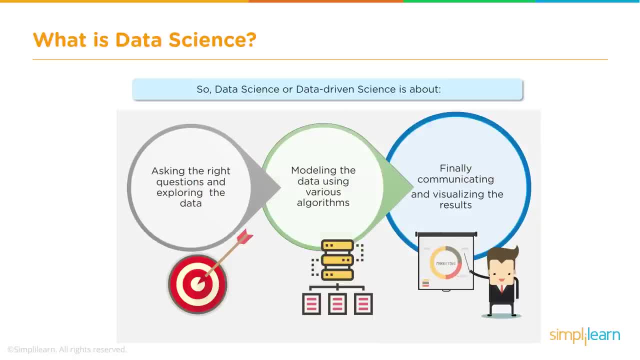 And then you come out with the final results of this exercise, which includes visualizing the results and preparing a way to communicate the results to the concerned people. So it could be in the form of PowerPoint slides or it could be in the form of a PowerPoint. 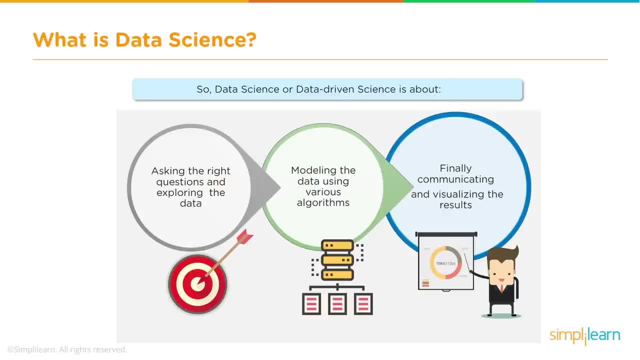 dashboard, which is basically what we call as a visualization, And so all the insights that have been gathered through this exercise, that has to be communicated in a proper way, in an easy to understand way, which is again a key part of this whole exercise: communicating. 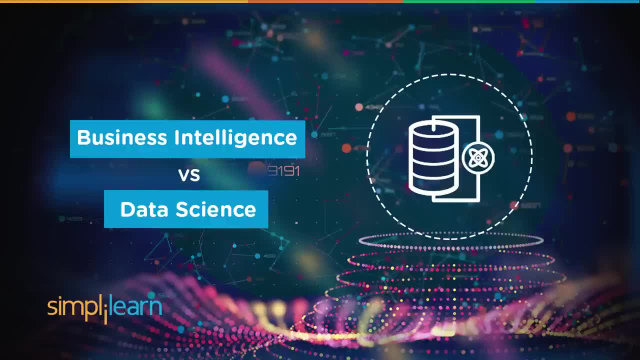 the results. So let's now talk about the difference between business intelligence and data science. Now, business intelligence was one of my favorite things about data science. It was one of my favorite things about data science. It was one of the initial phases where people started. 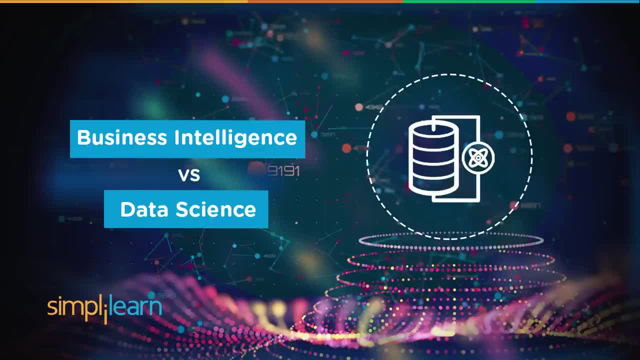 making or wanted to make some sense out of data. So, for some of you who may not be aware, there were multiple phases of this IT revolution. So initially there was all automations. You had automation of your selling process, manufacturing process. You had your ERP systems, your CRM. 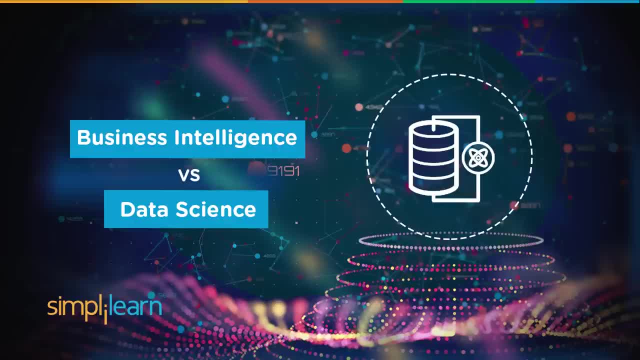 systems and so on, which are basically enterprise resource planning and customer relationship management, ERP and CRM, And all these enterprise applications were generating a lot of data. So then people started saying that, okay, we need to understand or get some information out of this data. So 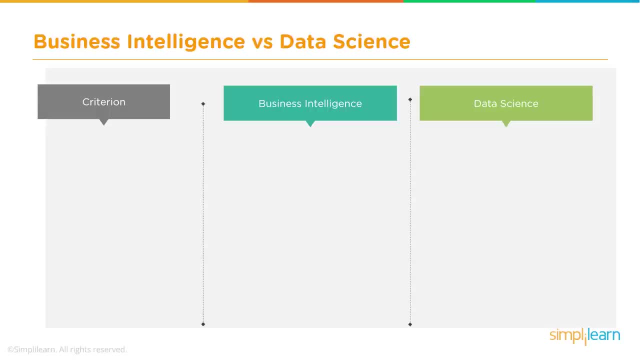 that's how business intelligence started. So if we take from a data source perspective, let's compare these from with each of these criteria. The criteria are: what is the data source, What is the method, What are the skills and what is the focus. And if we compare business, 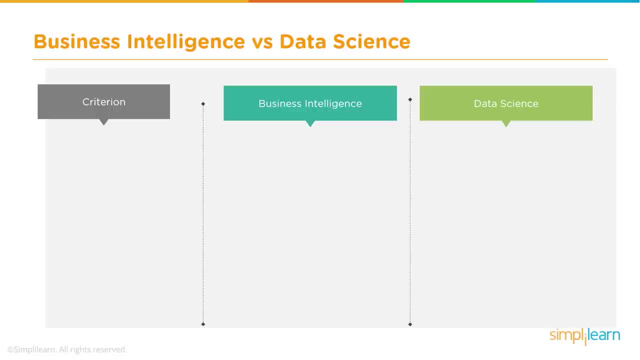 intelligence with data science. this is how it looks. As far as the data source is concerned, business intelligence was primarily using structured data. So you had all your enterprise applications like ERP, CRM and so on, and they were working out of pretty much RDBMS relational database. 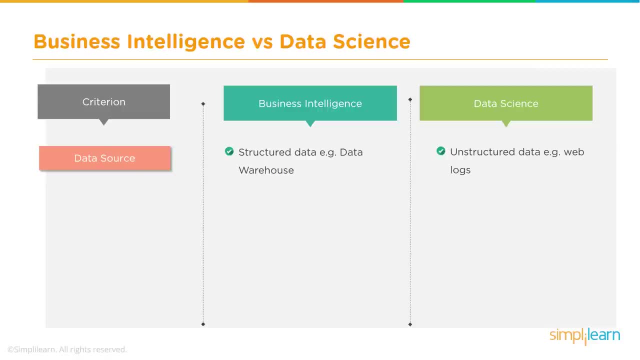 management systems like Oracle or MS SQL, MySQL and so on. So all this data was structured in neat form, form of tables, rows and columns, And then they were all brought into a centralized place because, remember, these were still different applications. So 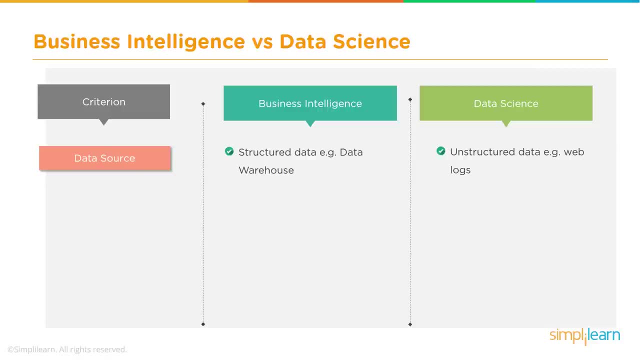 they were working off different databases in silos. So if you wanted to get a combined view, you needed to create what is known as a data warehouse and bring all this data together and then look at it in a uniform way. So this is what 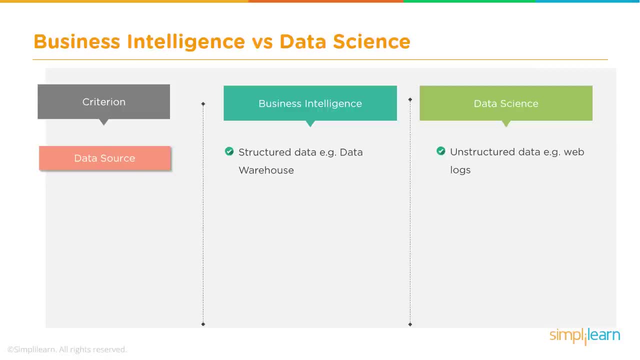 business intelligence was doing Pretty much. it was structured data and it had reports and dashboards. So that was pretty much what was there in business intelligence. Now, with the data science, in addition to structured data, we also use a lot of unstructured data. Example: web logs. 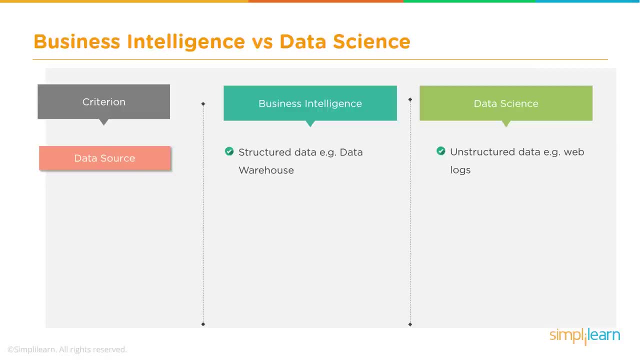 or comments. If we are talking about customer feedback. there is a structured part. there is an unstructured part where people write free text. Data science includes that as well and brings everything and then performs analysis. So, data source wise. that is the difference. 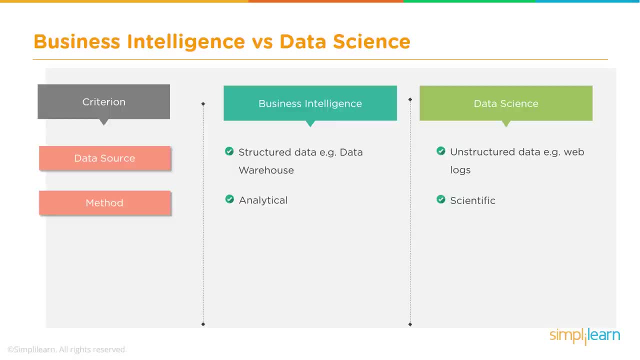 Now methods In business intelligence. pretty much it is analytical in the sense that, okay, you have some data, we are just trying to present the truth and mostly what has happened- Historical data, That's it. In case of data science, we go beyond that. we go deeper in terms of finding why a certain 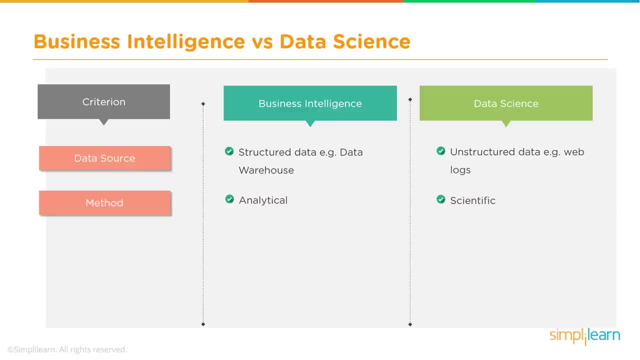 behavior has occurred and also go beyond just providing a report. There is a deeper statistical analysis that is done, That is what is the scientific part, And deeper insights are gathered, not just reporting. So that's from a method perspective, From a skills perspective. 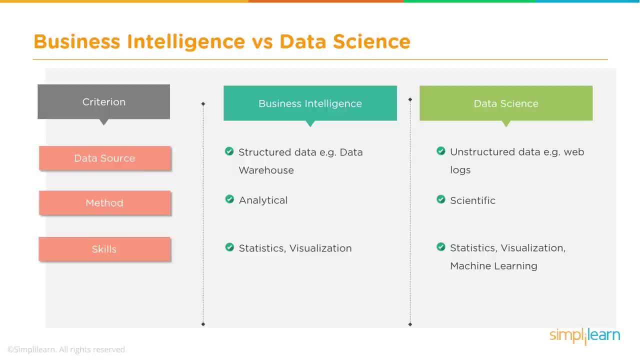 business intelligence needs a little bit of statistics but more of visualization, because they primarily consisted of dashboards or they primarily consist of dashboards and reports, Whereas in data science, the visualization, of course, is there, but there is a lot more of statistics involved. 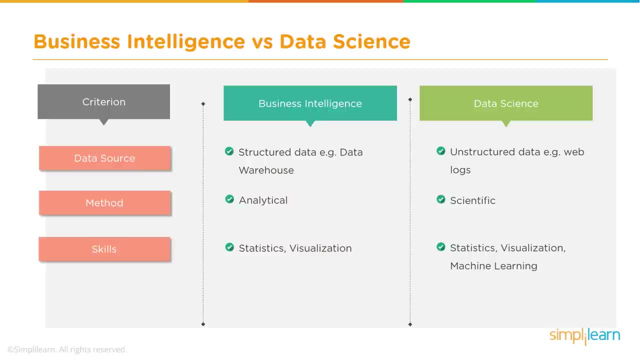 because we are looking at things like correlation. We are looking, for example, if we perform machine learning, we try to do regression, try to predict what will be the sales maybe in the future, and so on and so forth. So it is much more involved in case of data science. 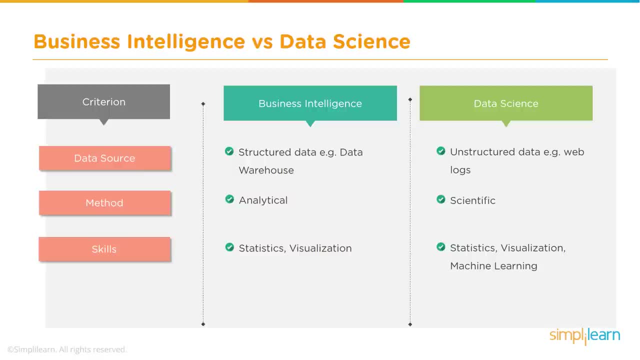 compared to business intelligence. The skills are many more compared to business intelligence. And, last but not least, what is the focus? Focus of business intelligence is pretty much historical data, So the sales have happened. based on the sales till today, You try to come up with a report. 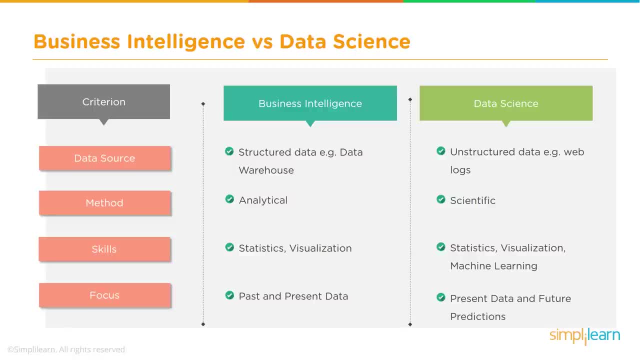 What was my sales? Maybe for this whole year, or maybe for the last five years, and so on and so forth. In data science you take historical data, but you also combine that with maybe some other required information and you also try to predict the future. 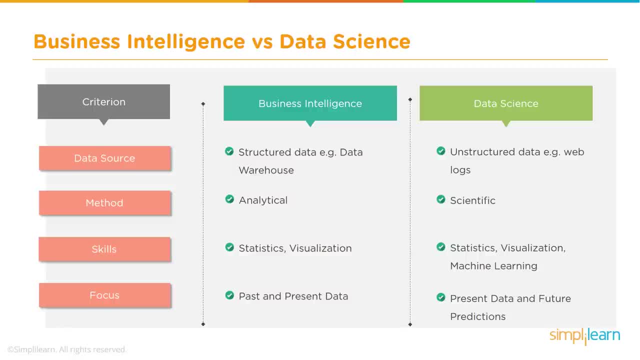 So we try to extrapolate maybe the sales and say: okay, sales as of now, as of today, this is sales is 5 million And if we, based on the, the historical data, we say, oh, this is 1 million. 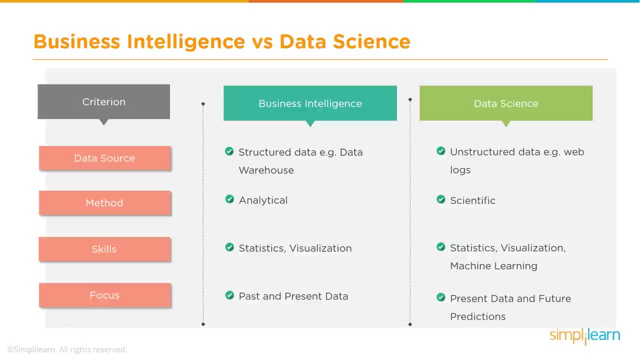 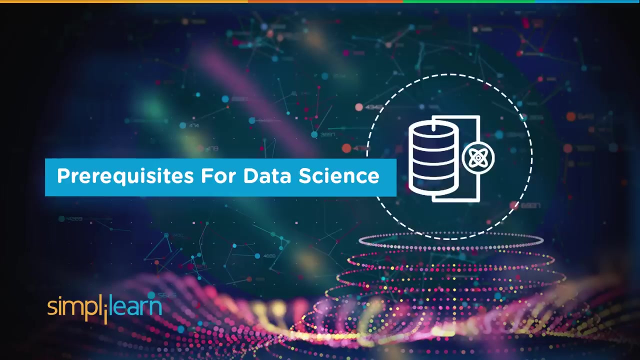 information, we see that sales increase on a maybe, I don't know- monthly basis: 10%. That is what history says. So our sales for next month will be this much right. So that is the focus of data science. It goes beyond just reporting. So what are the prerequisites for data science? There are: 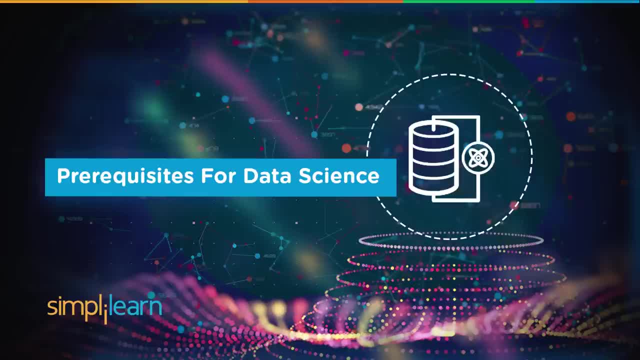 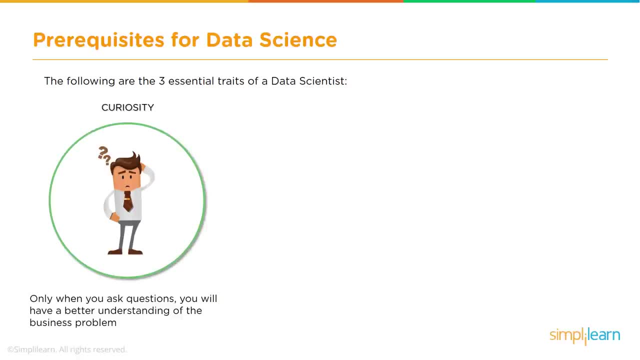 three essential traits required for to be a data scientist. One is curiosity. You need to be able to ask questions. The first step in data science is asking questions. What is the problem we are trying to solve? If you ask the right question, only then you'll get the right answer. Very often, 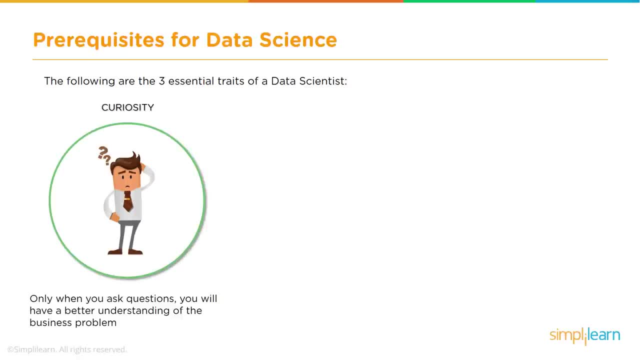 this is a very crucial step, where a lot of data science projects fail because you may be asking the wrong question And then, obviously, when you get the answer, that's not the answer you're looking for. So it is very important that you ask the right question. Needless to say, then, the 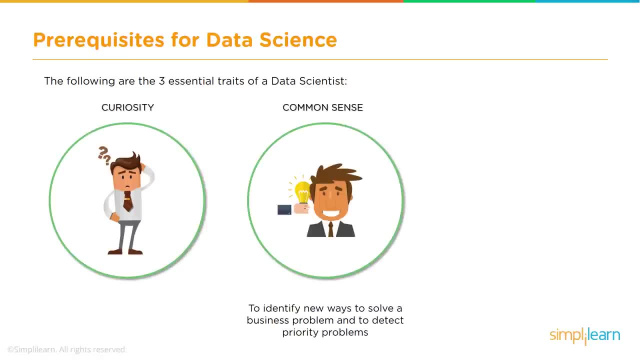 second part, or the second trait is common sense. So you need to be creative, you need to come up with ways to use the data that you have and try to solve the business problem on hand. In many cases, you may not have all the data that you need. In many cases, the data may be incomplete, So that 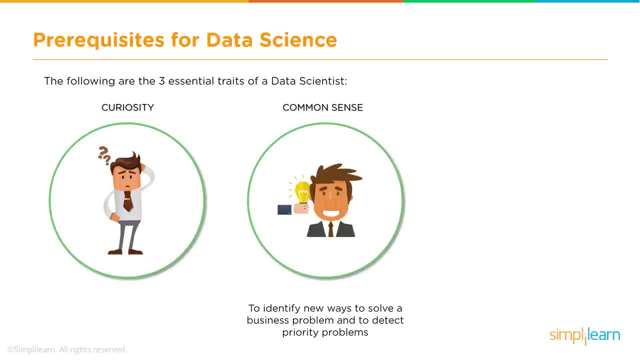 is where you need to come up with ways. what are the best ways to fill these gaps wherever this is missing, And that's where common sense comes into play. Last but not least, after doing all this analysis, if you're unable to communicate the results and the right to be a data scientist. 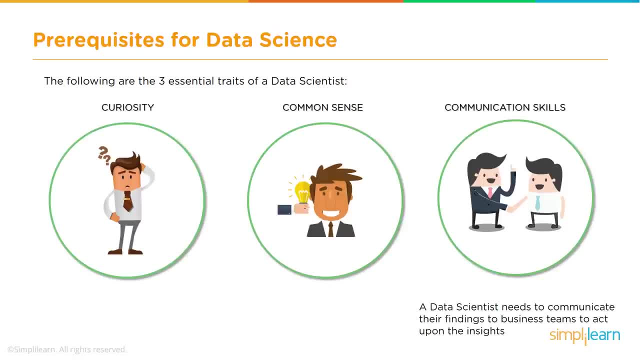 the whole exercise will fail. So communication is a key trait for a data scientist. Maybe technically you may be a genius, but then if you are unable to communicate those results in a proper way, once again that will not help. So these are the three main traits. 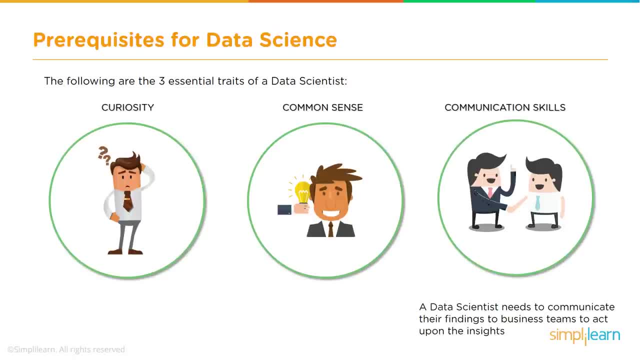 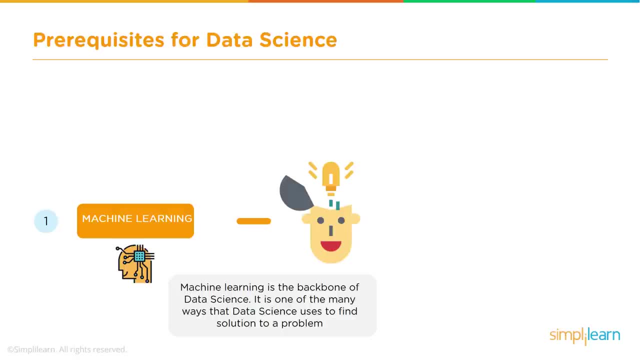 curiosity, common sense and communication skills. In a way, you can say these are the three Cs. Okay, so what are the other prerequisites? First one, so machine learning. Machine learning is the backbone of data science. Data science involves quite a bit of machine learning in addition to 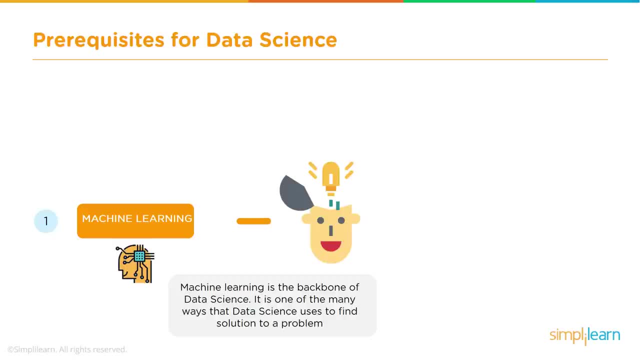 the basic statistics that we do. So a data scientist needs to have a good hang, or need to be very good, at data science. The second part is modeling. So modeling is also a part of machine learning in a way, but you need to be good at identifying what are the algorithms that 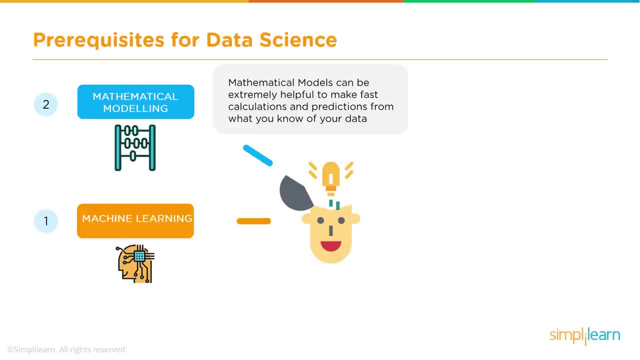 are most suitable to solve a given problem, What models can we use And how do we train these models, and so on and so forth. So that is the second component. Then statistics: Statistics is like the core foundation of data science, So you need to understand. 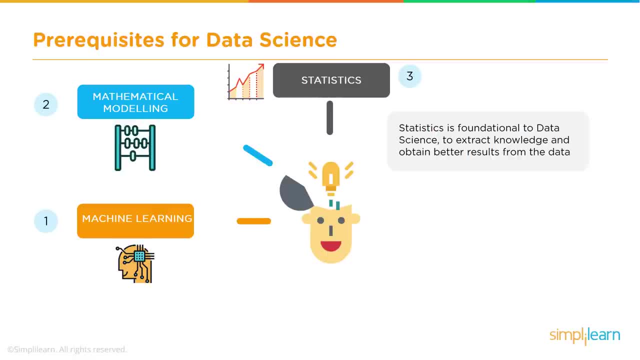 statistics, and you need to have a good hang of statistics in order to be a good data scientist, And this will also help in getting good results. Programming is, to some extent, required. At least some program or the other would be required as a part of executing a data science. 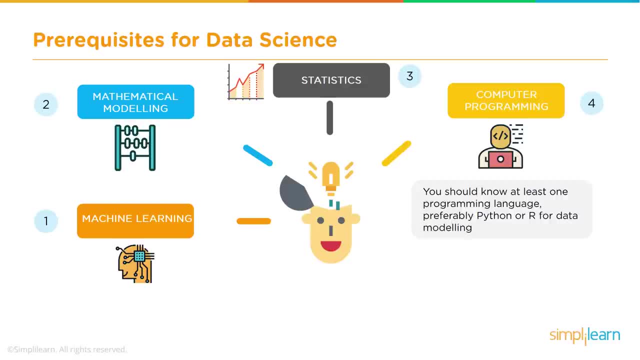 Project. The most common programming languages are Python and R. Python, especially, is becoming a very popular programming language in data science because of its ease of learning, because of the multiple libraries that it supports for performing data science and machine learning, and so on. So 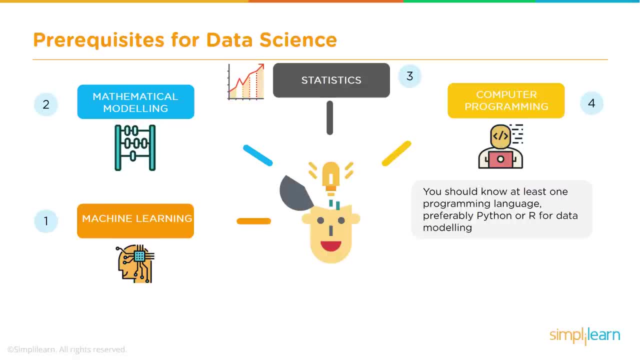 Python is by far one of the most popular languages in data science. If any one of you is is wanting to learn a new language, that should be Python. And then, of course, you need to understand databases, how databases work and how to handle databases, how to get data out of databases, and so on. So these are some of the key components. 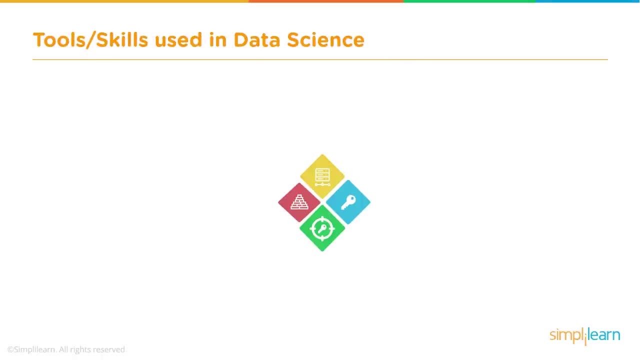 of data science. Now coming to the tools and skills that are used in data science. These are some of the skills. from a language perspective, It is Python or R And, from a skills perspective, in addition to some of the programming languages, it would help if you have a good knowledge or good understanding of statistics. 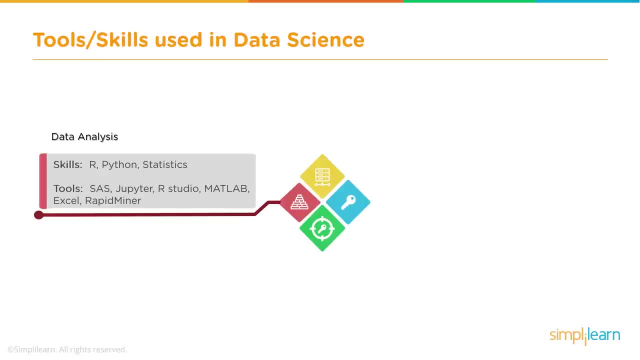 And what are the tools that are used in data analysis? SAS is one of the most popular tools. It's been there for a very long time and that's the reason it is very popular And, however this is compared to most of the other tools, It is a proprietary software, whereas Python and R 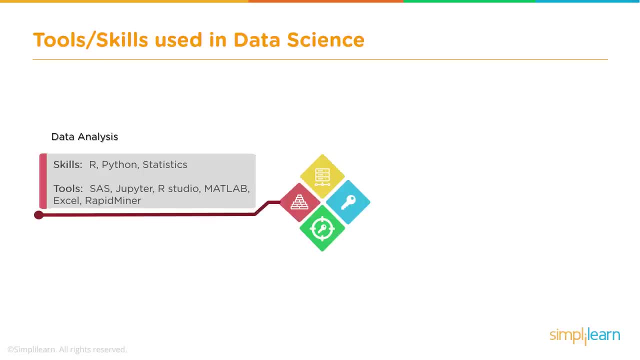 are mostly open source. The other tools are like Jupyter Notebooks. you have RStudio. These are more development environments and development tools. So Jupyter Notebooks is an interactive development environment. Similarly, RStudio is for performing or writing R code and performing analytics and performing data analysis and 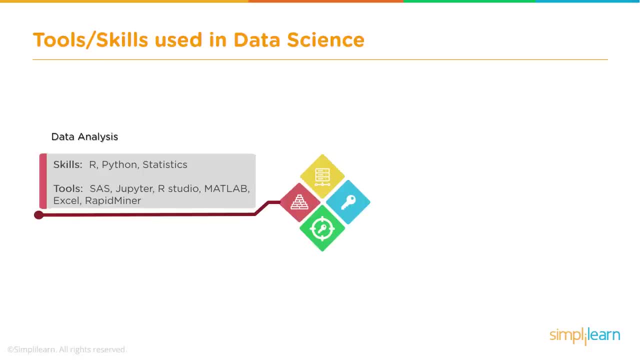 machine learning activities You can perform in RStudio. It has a very nice UI and initially R was not so popular, primarily because it did not have the interface. And RStudio is a relatively new edition And after the advent of RStudio R became extremely popular. And there are other tools like MATLAB And, of course, 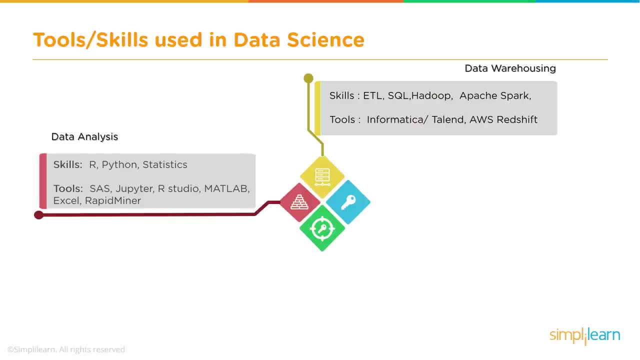 some people do with Excel as well. As far as data warehousing is concerned, some of the skills that are required are ETL. So in order to extract data and transform load, ETL stands for extract, transform load. So you have data in the databases, like your ERP system or. 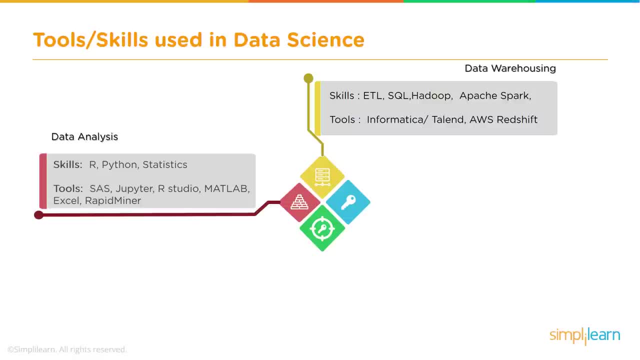 your RAM system. You need to extract that and then do some transformations and then load it into your warehouse so that all the data from various sources looks uniform. Then you need some SQL skills, which is basically querying the data, writing SQL queries. Hadoop is another. 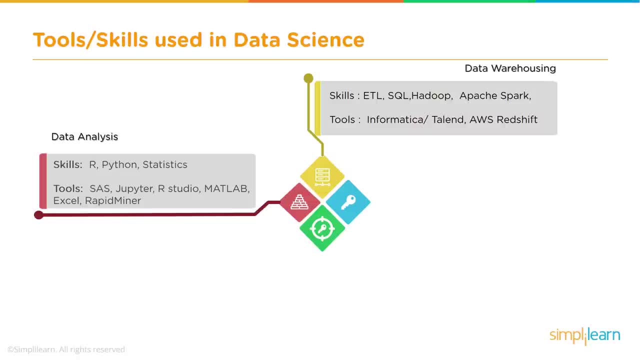 important skill, especially if you're handling large amounts of data, And also one of the specialties of Hadoop is it can be used for handling unstructured data as well. So it can, you know, be able to do a lot of things. So it can be used for handling unstructured data as well. So it can be used for handling unstructured data as well. So it can be used for handling unstructured data as well. So it can. 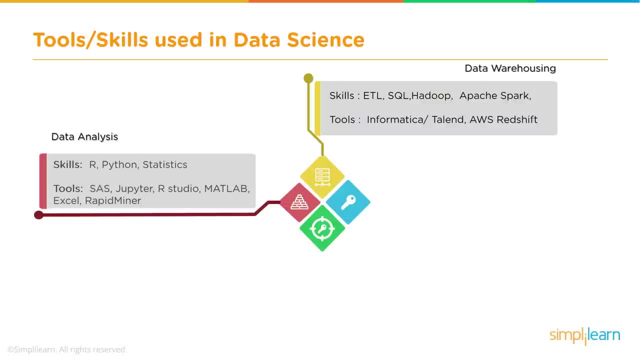 be used for large amounts of structured and unstructured data, Then Spark is an excellent computing engine for performing data analysis or machine learning in a distributed mode. So if you have a large amount of data, the combination of Spark and Hadoop can be extremely powerful. 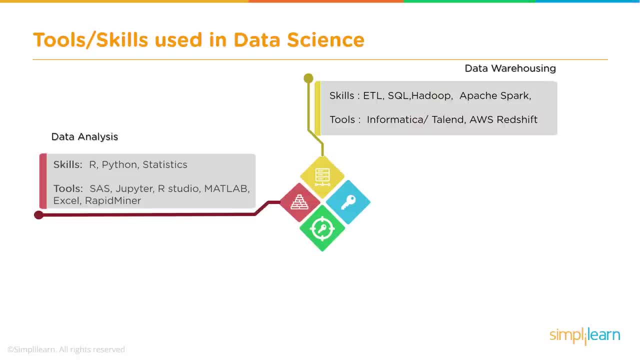 So you store your data in Hadoop HDFS and use Spark as your computation engine. It works in a distributed mode similar to Hadoop, in like a cluster, So that those are excellent skills for data warehousing And there are some standard tools that are available. 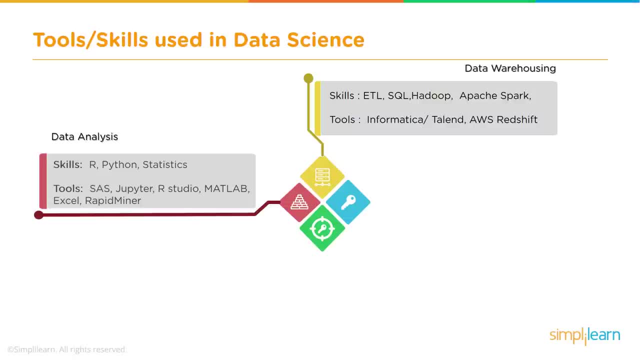 like Informatica, Data Stage Talent and also AWS Redshift. If you want to do some on the cloud, I think AWS Redshift is again a good tool. Data visualization tools. For data visualization. some of the skills that would be required are, let's say, R. R provides some very good. 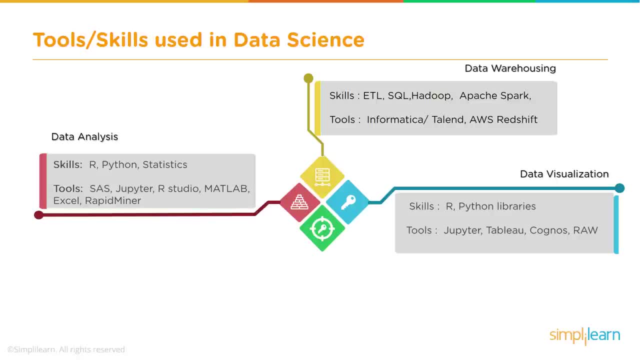 visualization capabilities, especially for developing during development. And then you have Python libraries, Matplotlib and so on, which provides very powerful visualization capabilities, And that is from skills perspective, Whereas tools that can be used are: Tableau is a very, very popular visualization tool. Again, that's a proprietary tool, So it's a little expensive. 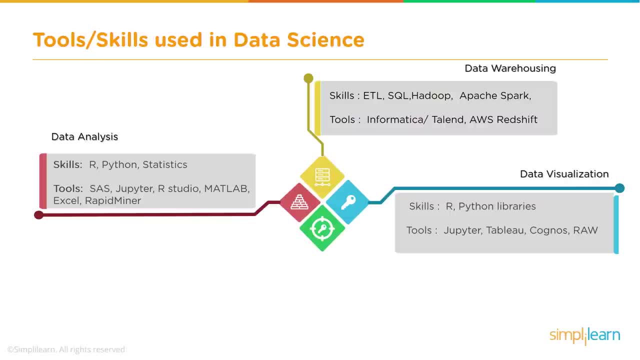 maybe, but excellent capabilities from a visualization perspective. Then there are tools like Cognos, which is an IBM product, which provides very good visualization capabilities as well. And then, coming to the machine learning part of it, the skills required. there are Python, which is more 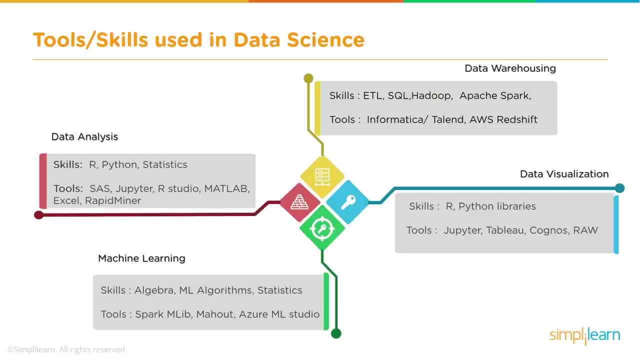 for the programming part, And then you will need some mathematical skills like algebra, linear algebra especially, and then statistics and maybe a little bit of calculus and so on. And the tools that are used for machine learning are Spark, MLlib and Apache. 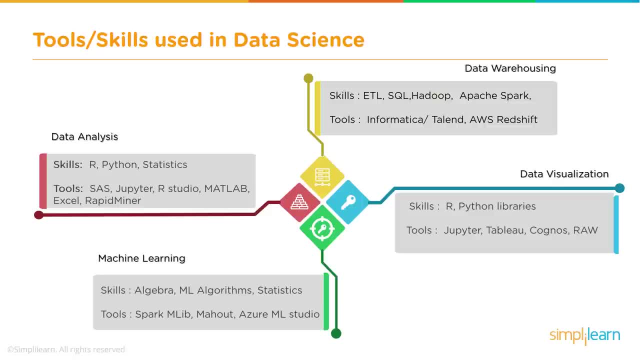 Mahout and on cloud. if you want to do something, you can use Microsoft Azure ML Studio as well. So that's it for this video. Thank you so much for watching and I'll see you in the next one. Bye, bye. 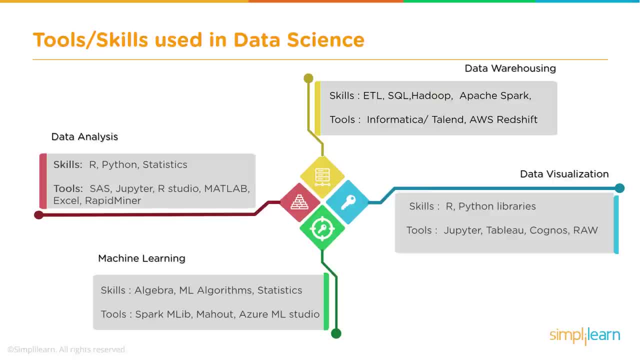 So these are by no means an exhaustive list. There are actually many, many tools and probably a few more skills also maybe there, but this is. this gives a quick overview, like a summarizing of summarization of the tools and skills. Now moving on to the life. 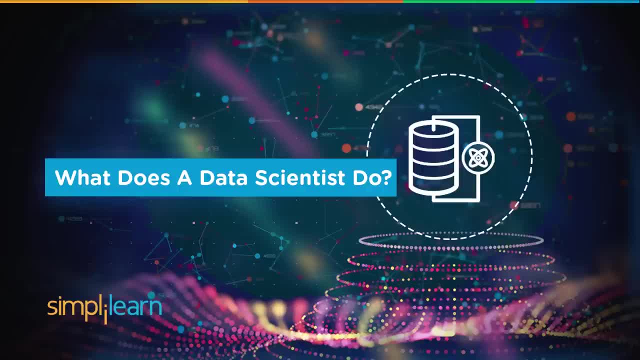 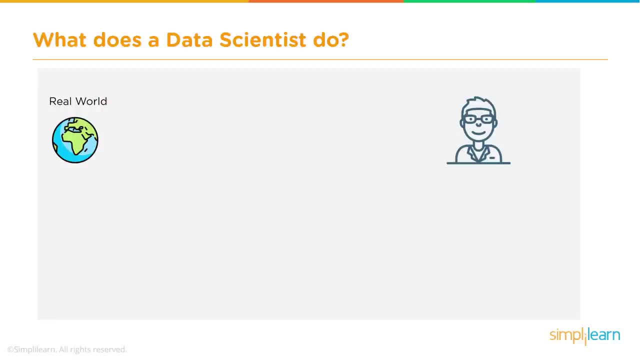 of a data scientist. what does a data scientist do during the course of his work? So let's see So: typically, a data scientist is given a problem, a business problem that he needs to solve, And in order to do that, if you remember from the previous slide, he basically asks the question: 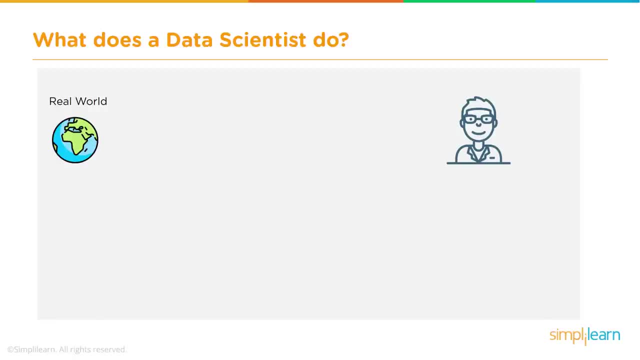 as to what is the problem that he needs to solve. So that is the first thing. He has got the problem. Then the next thing is to gather the data that is required to solve this problem. So he goes about looking for data from anywhere. It could be the enterprise. Very often the data is not provided in. 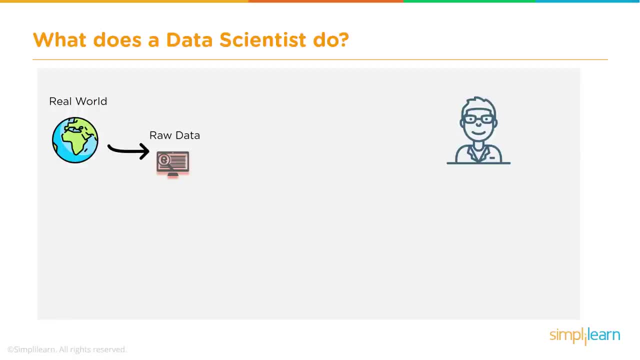 the nice format that he would like to have it or we would like to have it. So first step is to get whatever data that is possible- What is known as raw data, in whatever format. So it could be enterprise data, It could be. 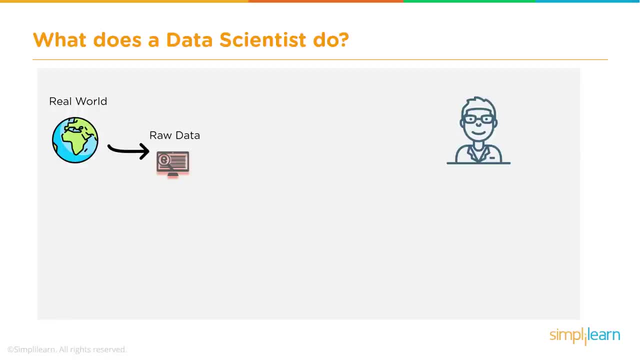 there is a probably a requirement to go and get some public data in some cases. So all that raw data is collected and then that is processed and analyzed and in prepared into a format in which it can be used And then it is fed into the analytics system. be it a mission. 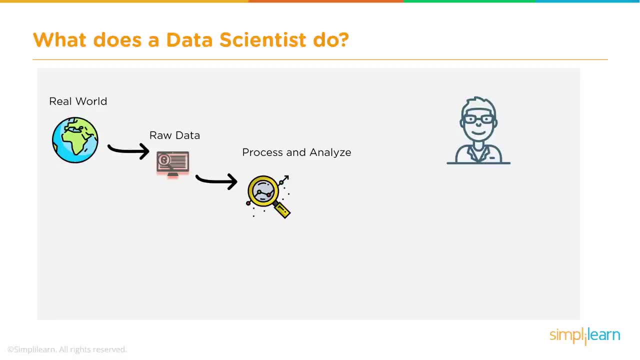 learning algorithm or a statistical model And we get the output And then he puts these output in a proper format for presenting it to the stakeholders and communicating those insights or the results to the stakeholders. So this is a very high level view of like a day in. 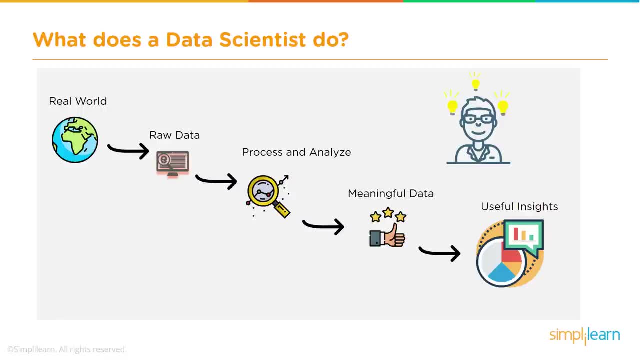 the life of a data scientist. So gathering data, raw data, performing some quick analysis on that and maybe processing or manipulating this data to bring it into a certain good format so that it can be used for the analysis, feeding this into that analysis system that has been designed be it. 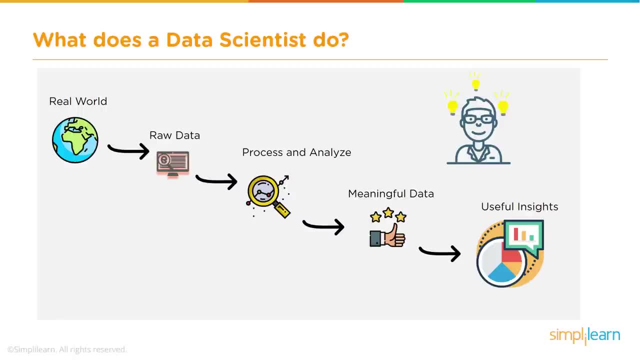 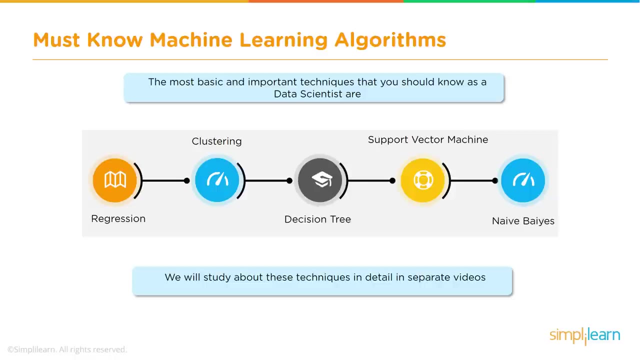 mathematical models, machine learning models, and then get the results, the insights, and then present it in a nice way so that the stakeholders can understand. How about machine learning algorithms? So let's see what are the various machine learning algorithms that would be required. 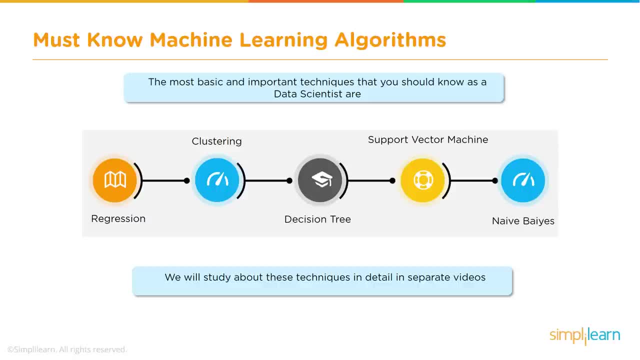 for a data scientist. So these are a few of the algorithms. Again, there's not actually a lot of information about data scientists, But there's a lot of information about the algorithms that might be required for a data scientist. So there's a lot of information about. 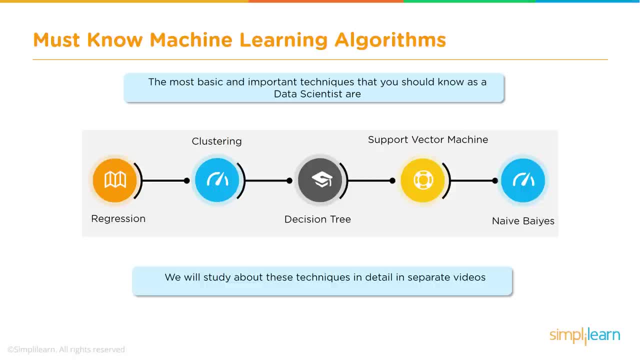 exhaustive list we have. regression is one of the supervised learning models or techniques. so in case of regression you try to, let's say, come up with a continuous number. so the difference between regression and, let's say, a classification is that in case of classification, those are discrete. 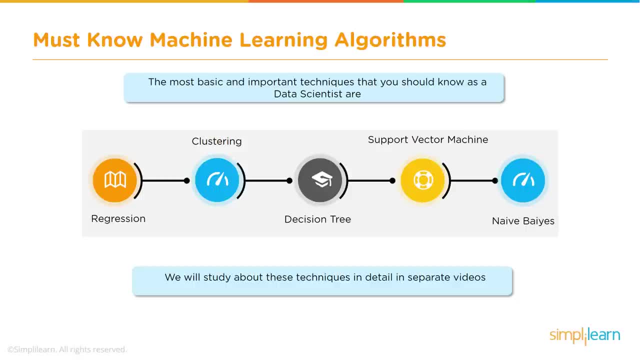 values, whereas here we are talking about regression, where you, let's say, you are trying to predict the temperature, which is a continuous value, or the share price, which is a continuous value. so that is regression. so you need to know what is regression, how to perform regression, and we need to 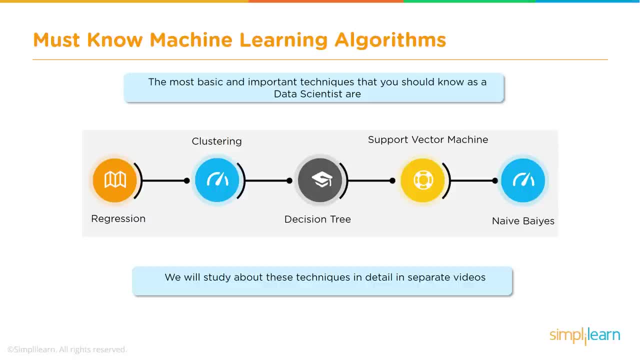 understand clustering. so clustering is one of the unsupervised learning techniques. in this case there is no label data that is available and you get some data and then you want to put this into some shape so that you can analyze it and you try to make sense out of it. let's say you have 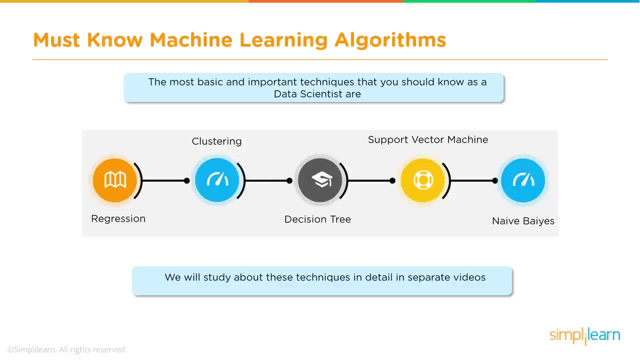 one example, as you have a list of cricketers and they have not been marked as bowlers and batsmen or all-rounders or whatever right, so you just have their names and maybe how many runs they scored, how many wickets they have taken and so on, but there is no readily available information saying 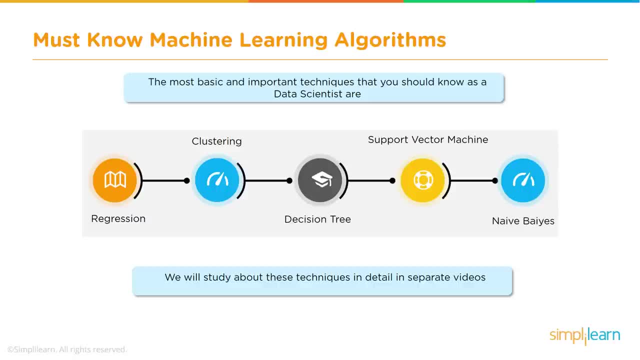 that, okay, this person is a batsman, this person is a bowler, and so on. so i'm talking about cricket. hopefully most of you are familiar with the game of cricket. so how do we find out? so then we put this into a clustering mechanism and then the system will say that: 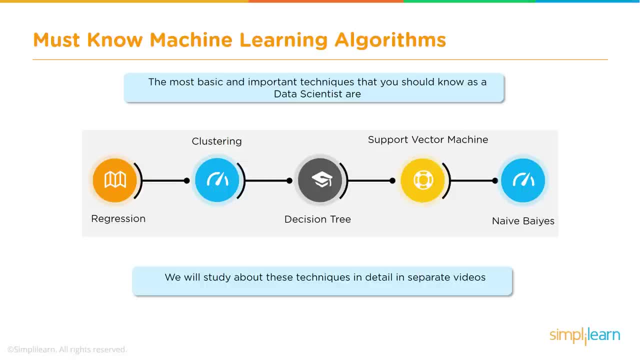 okay, these are the people who are all- who have all scored good amount of runs, so they belong to one cluster. these are all the people who have taken good amount of wickets, so they belong to one cluster. and maybe here are some people who have taken good amount of wickets and they have made 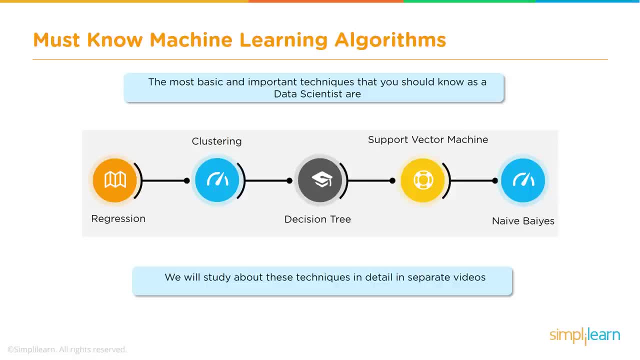 good amount of runs, so they may be belonging to one group, and then we take a look at it and then we label them as okay, people who have all together and those who have, you know, scored many runs they are. we label them as batsmen, people who have taken a lot of wickets, we label them as bowlers, and 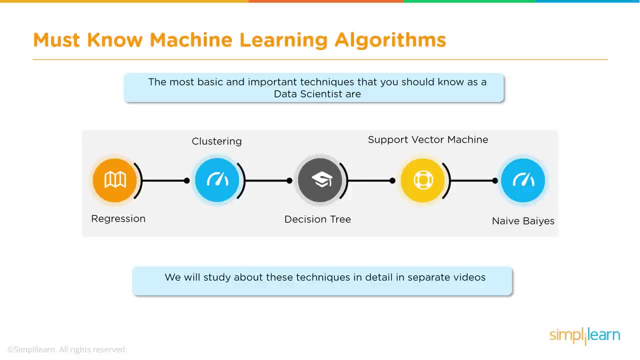 people who have taken a good amount of wickets and also made some good runs. we label them as all-rounders. but the system will just say, okay, this is cluster one, cluster two, cluster three- the names we give the human beings have to give the names. now decision tree is used for what is? 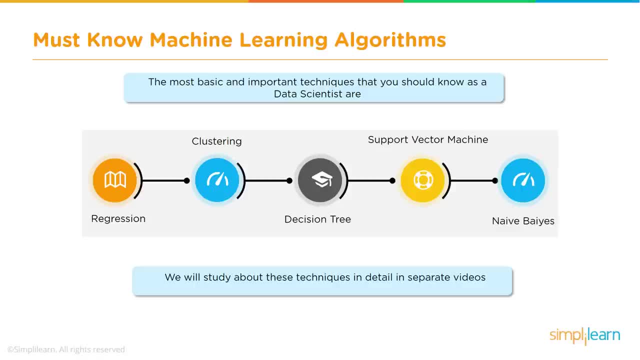 known as classification primarily. it can also be used for regression, but by and large it is used for classification, and here again it's a very logical way in which the algorithm goes about classifying the various inputs. one of the biggest advantages of decision tree is that it's very easy. 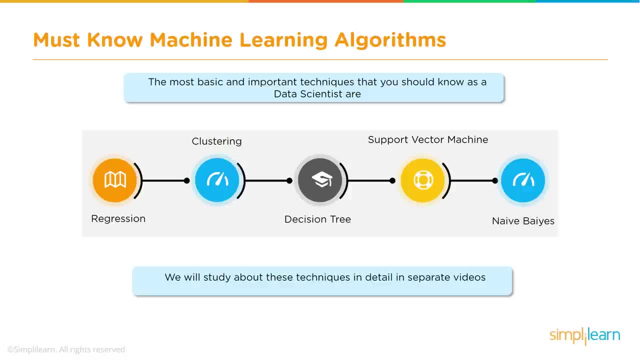 to understand and it's very easy to explain why a certain object has been classified in a certain way, compared to maybe, some of the other mechanisms like, say, support vector machines or logistic regression and so on. so that's the advantage of decision tree, but that is also very popular algorithm. then we have support vector machines, primarily for 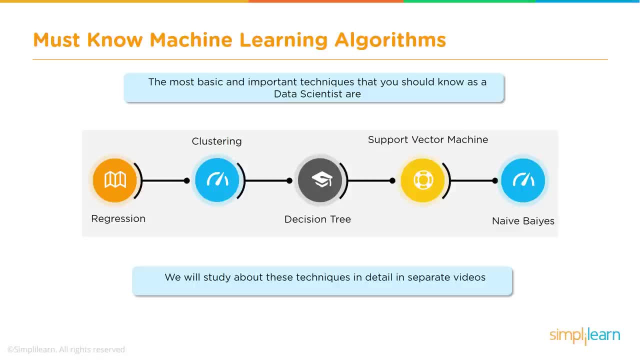 classification purpose. and then we have naive base. this is again a statistical probability based classification method. so these are a few algorithms. there are a few more that are not listed here, but there are some more algorithms as well and, by the way, there are more detailed or there are detailed videos about each of these algorithms available. you can check. 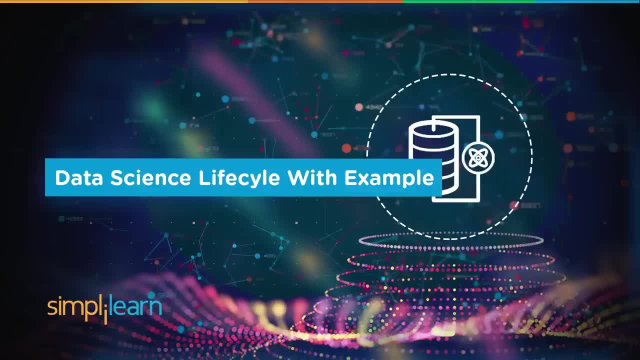 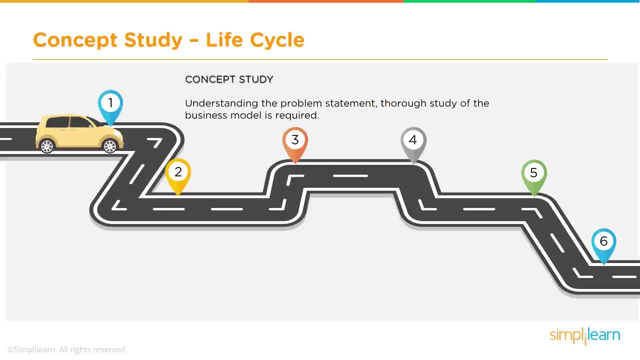 in the playlist. so now let's talk about the life cycle of a data science project. okay, the first step is the concept study. in this step, it involves understanding the business problem: asking questions, get a good understanding of the business model, meet up with all the stakeholders, understand. 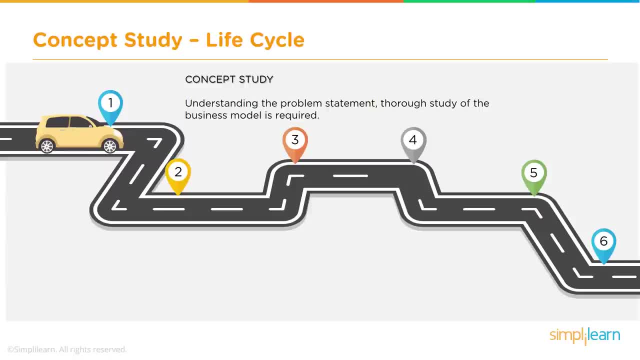 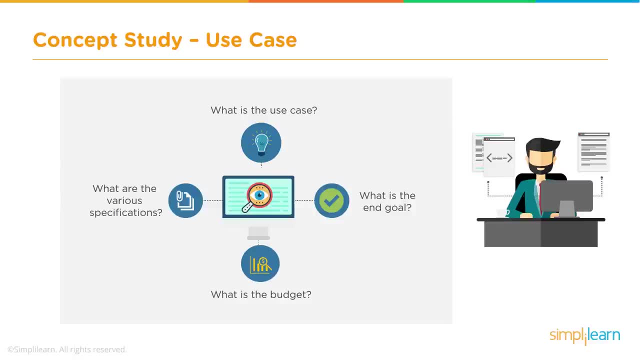 what kind of data is available. and then the second step is the concept study. so this is a part of the first step. so here are a few examples. we want to see what are the various specifications and then what is the end goal, what is the budget? is there an example of this kind of a problem that has been maybe solved earlier? 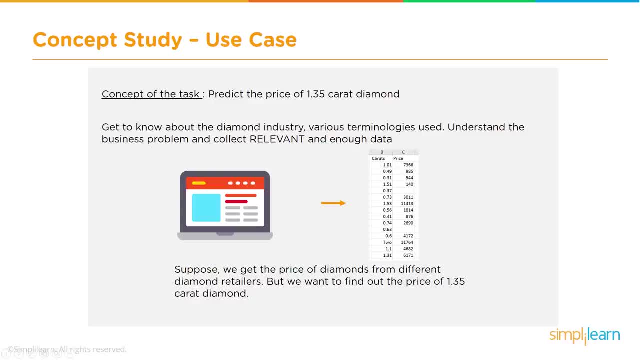 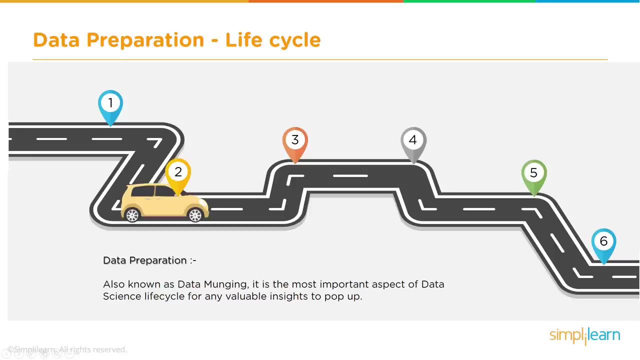 so all this is a part of the concept study, and another example could be a very specific one: to predict the price of a 1.35 carat diamond, and there may be relevant information inputs that are available and we want to predict the price. the next step in this process is data preparation data. 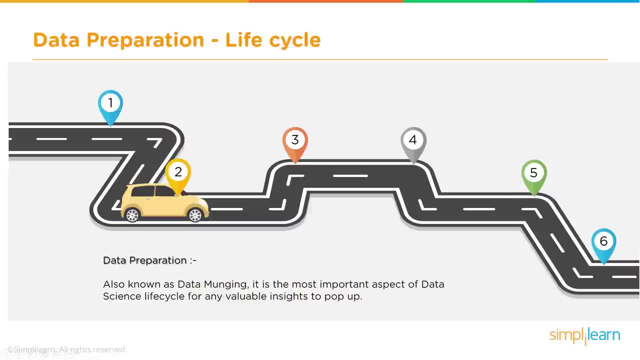 gathering and data preparation, also known as data munging, or sometimes it is also known as data manipulation. so what happens here is the raw data that is available may not be usable in its current format for various reasons. so that is why, in this step, a data scientist would explore the data he 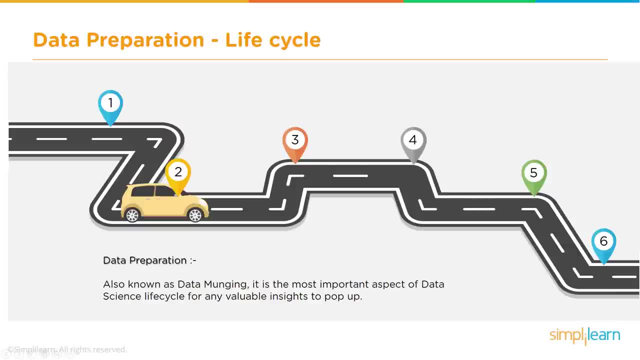 would look at some sample data, maybe pick. there are millions of records. pick a few thousand records and see how the data is looking. are there any gaps? is the structure appropriate to be fed into the system? are there some columns which are probably not adding value? may not be required for the. 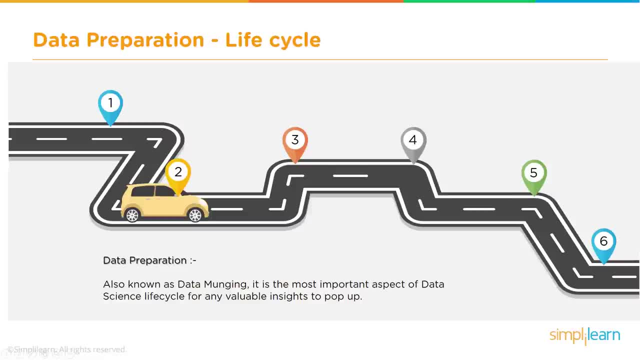 analysis. very often these are like names of the customers. they will probably not add any value or much value from an analysis perspective. the structure of the data: maybe the data is coming from multiple data sources and the structures may not be matching. what are the other problems? there may be gaps in the data. 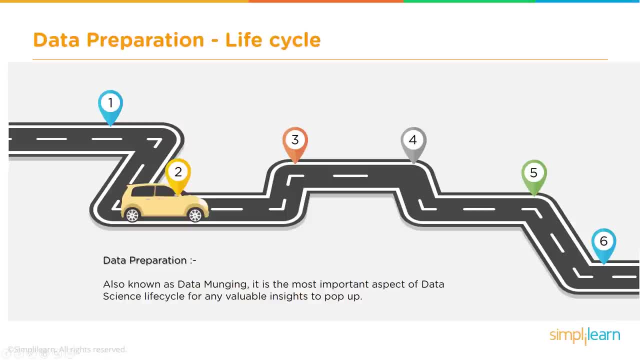 so the data, all the columns, all the cells are not filled. if you're talking about structured data, there are several blank records or blank columns. so if you use that data directly, you'll get errors or you will get inaccurate results. so how do you either get rid of the 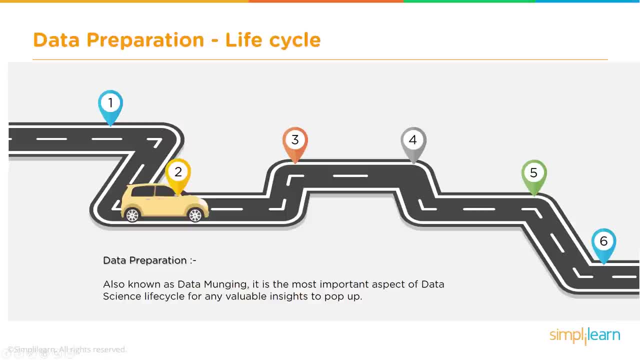 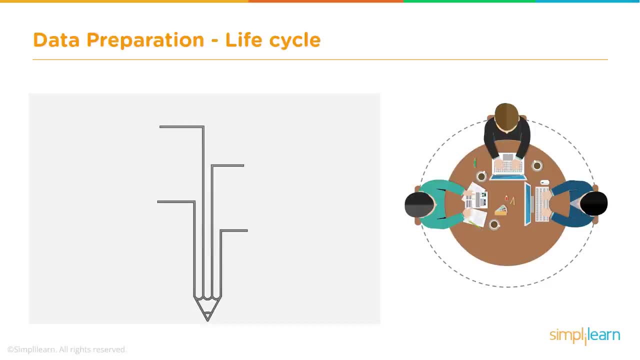 data or how do you fill this gaps with something meaningful. so all that is a part of data munging or data manipulation. so these are some additional sub topics within that, so data integration is one of them. if there are any conflicts in the data, there may be data may. 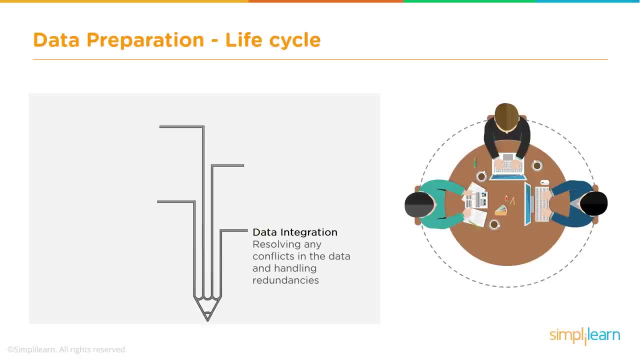 be redundant. yeah, data resident redundancy is another issue there may be. you have, let's say, data coming from two different systems and both of them have customer table, for example, customer information. so when you merge them, there is a duplication issue. so how do we resolve that? so 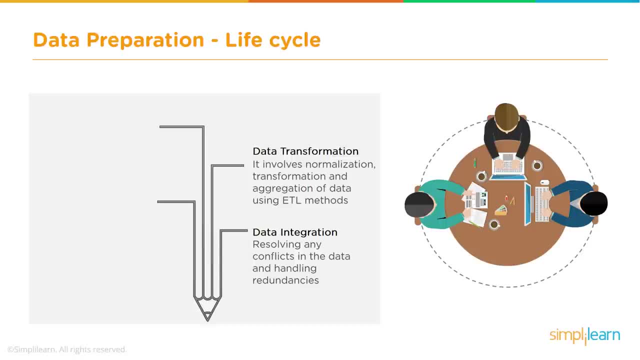 that is one data transformation. as i said, there will be situations where data is coming from multiple sources and then when we merge them together they may not be matching. so we need to do some transformations to make sure everything is similar. we may have to do some data reduction. 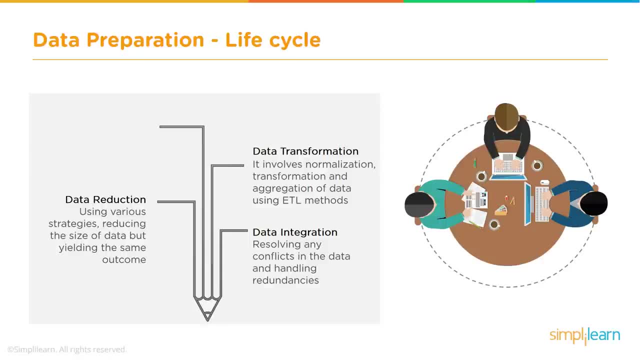 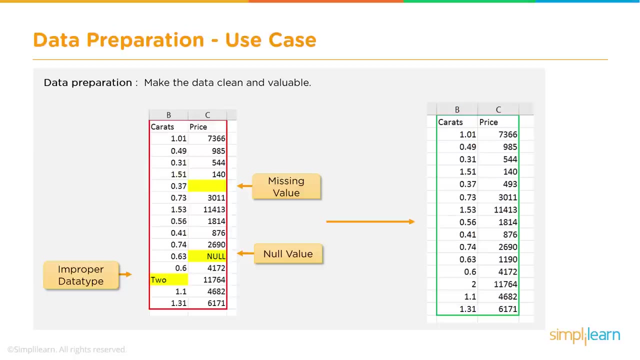 if the data size is too big, you may have to come up with ways to reduce it meaningfully without losing information. then data cleaning. so there will be either wrong values or null values, or there are missing values. so how do you handle all of that? a few examples of very specific stuff. 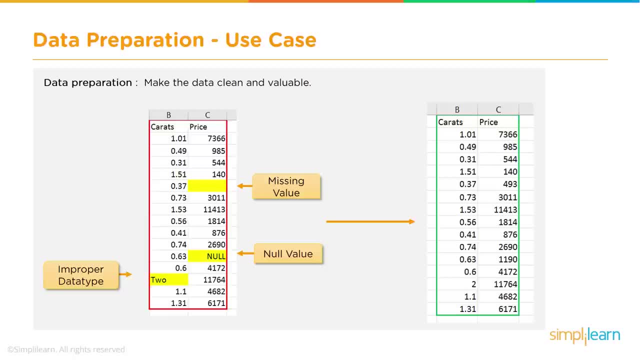 so there are missing values. how do you handle missing values or null values here? in this particular slide, we are seeing three types of issues. one is missing value, then you have null value. you see the difference between the two right. so in the missing value there is nothing, blank null. 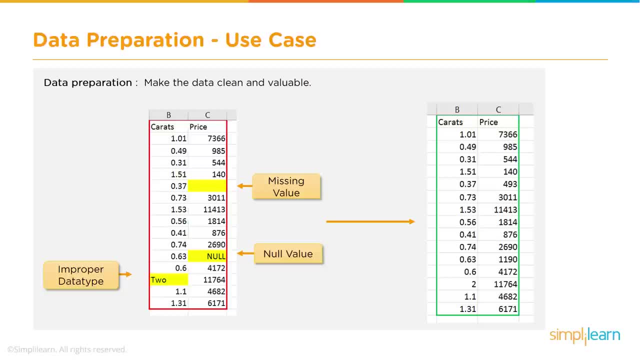 value, it says null. now, the system cannot handle if there are null values. similarly, there is improper data, so it's supposed to be a numeric value. so it's supposed to be a numeric value, so it's supposed to be a value. but there is a string or a non-numeric value. so how do we clean and prepare the data? 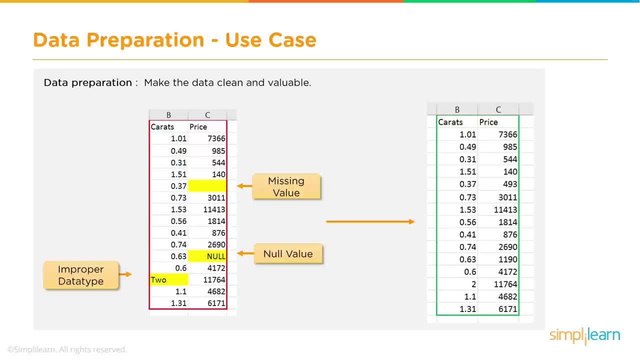 so that our system can work flawlessly. so there are multiple ways and there is no one common way of doing this. it can vary from project to project. it can vary from what exactly is the problem we are trying to solve. it can vary from data scientist to data scientist, organization to organization. so 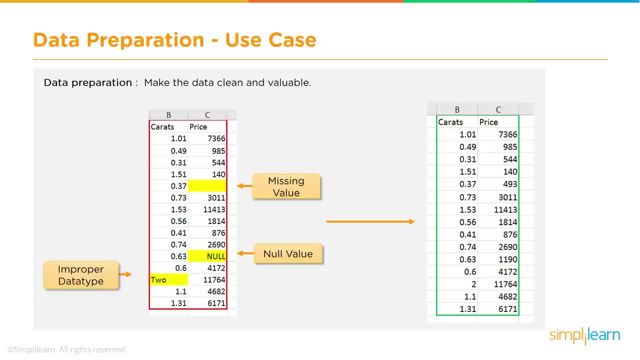 these are, like some standard practices people come up with and and, of course, there will be a lot of trial and error. somebody would have tried out something and it worked and will continue to use that mechanism, so that's how we need to take care of data cleaning. now, what are the various? 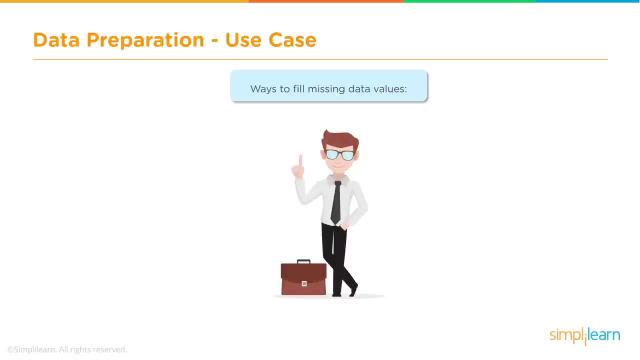 ways of doing. you know, if values are missing, how do you take care of that? now, if the data is too large and only a few records have some missing values, then it is okay to just get rid of those entire rows, for example. so if you have a million records and out of which 100 records don't have 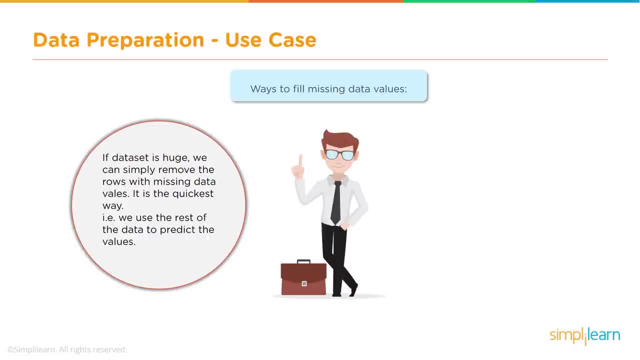 data. so there are some missing values in about 100 records. so it's absolutely fine because it's a small percentage of the data, so you can get rid of the entire records which are missing values. but that's not a very common situation. very often you will have multiple or at least a large number. 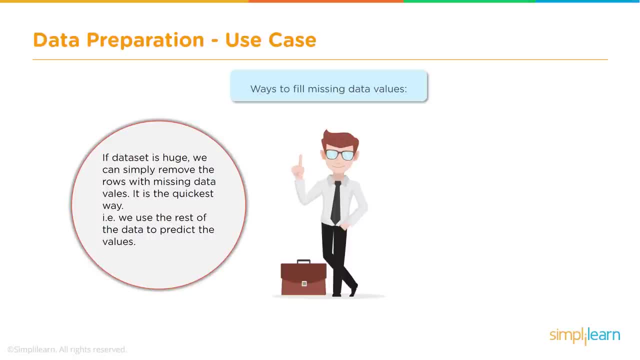 of a data set. for example, out of million records, you may have 50 000 records, which are like having missing values. now, that's a significant amount. you cannot get rid of all those records. your analysis will be inaccurate. so how do you handle such situations? so there are again multiple ways of. 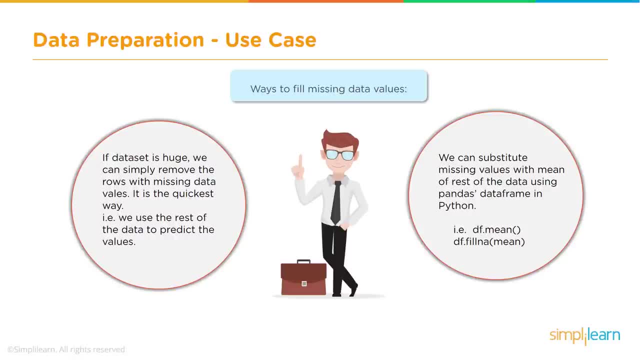 doing it. one is you can probably, if a particular values are missing in a particular column, you can probably take the mean value for that particular column and fill all the missing values with the mean value, so that first of all, you don't get errors because of missing values and second you 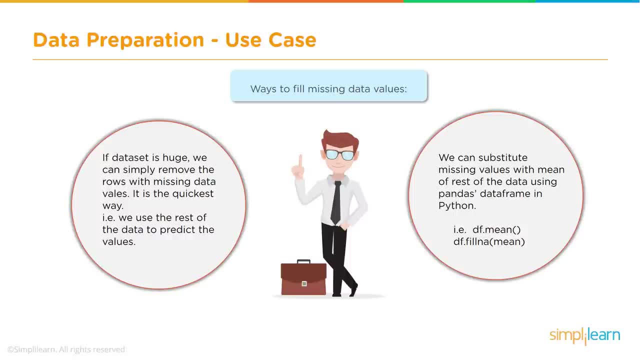 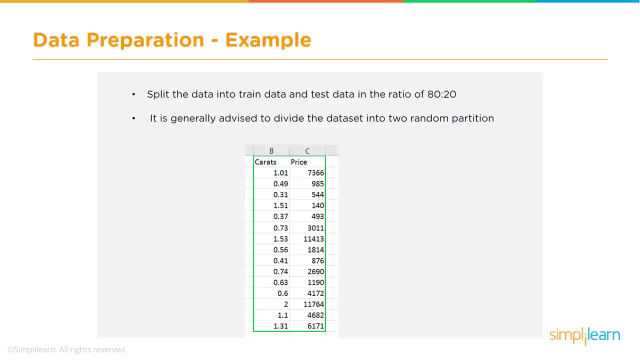 don't get results that are way off because these values are completely different from what is there. so that is one way. then few other could be, either taking the median value or, depending on what kind of data we are talking about, so something meaningful we will have put in there if we are doing some machine learning. 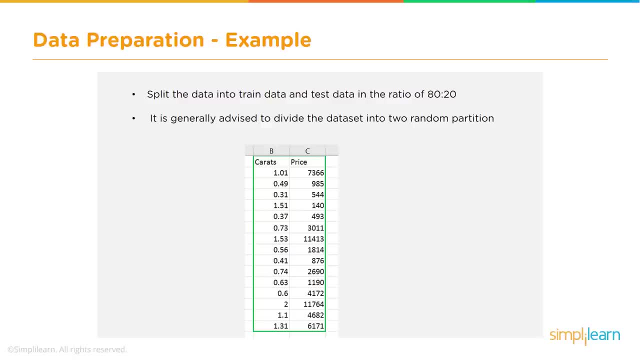 activity, then obviously, as a part of data preparation, you need to split the data into training and test data set. the reason being, if you try to test with a data set which the system has already seen as a part of training, then it will tend to give reasonably accurate results. 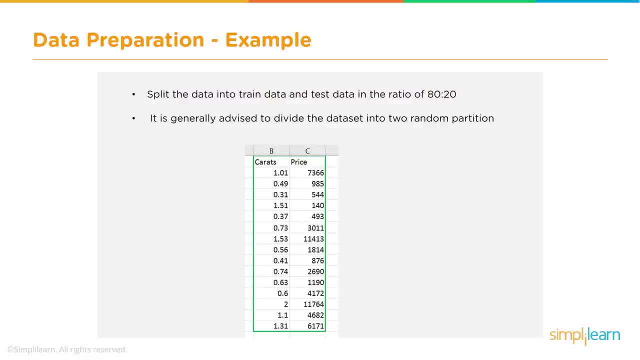 it has already seen that data and that is not a good measure of the accuracy of the system. so typically you take the entire data set, the input data set, and split it into two parts and again the ratio can vary from person to person, individual preferences. some people like to split it into 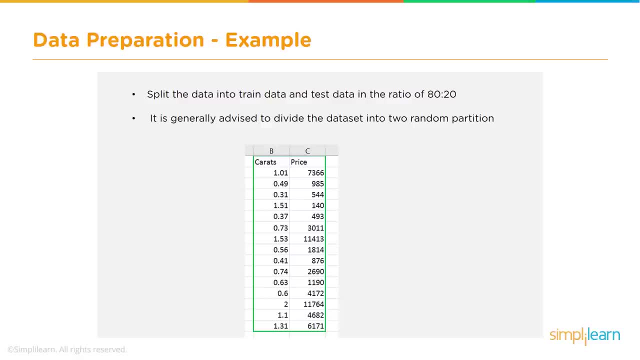 50, 50, some people like it as 63.33 and 33.3 is basically two-third and one-third, and some people do it as 80, 20, 80 for training and 24 testing. so you're the data. perform the training with the 80 and then use the remaining 20 for testing. all right, so that. 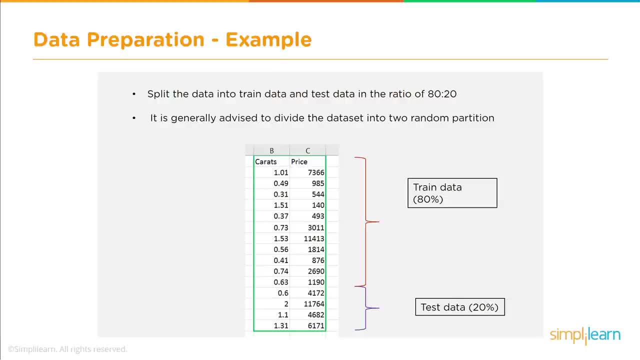 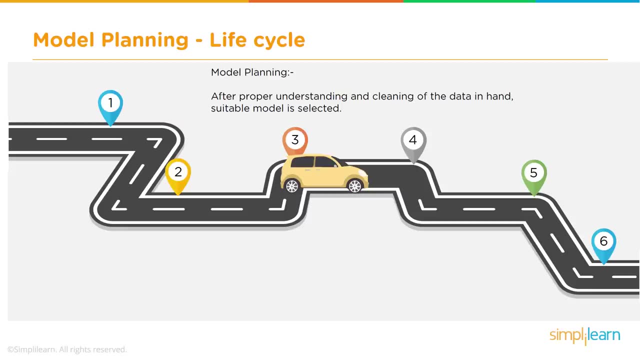 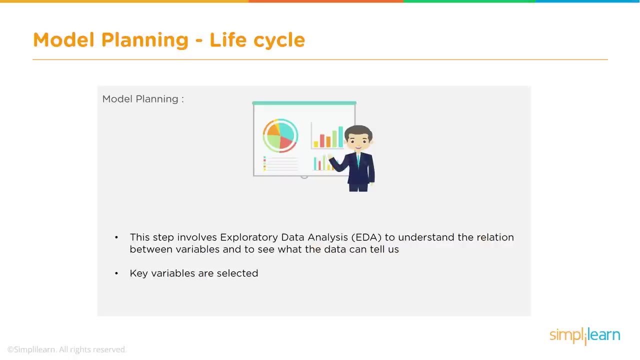 is one more data preparation activity that needs to be done before you start analyzing or applying the data or putting the data through the model. then the next step is model planning. now these models can be statistical models. this could be machine learning models. so you need to decide. 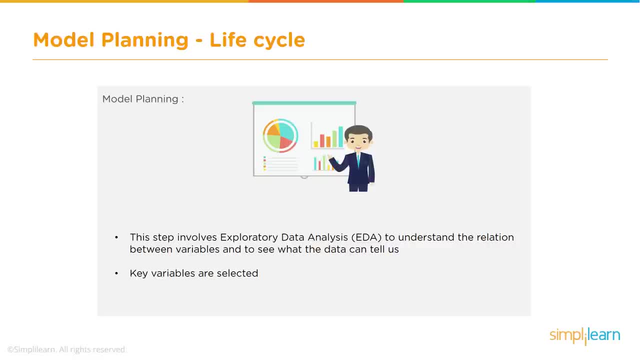 what kind of models you are going to use. again, it depends on what is the problem you're trying to solve. if it is a regression problem, you need to think of a regression algorithm and come up with a regression model. so it could be linear regression or if you. 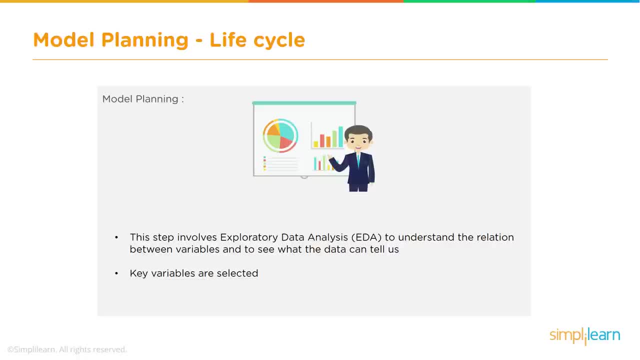 are talking about classification, then you need to pick up an appropriate classification algorithm, like logistic regression or decision tree or svm, and then you need to train that particular model. so that is the model building or model planning process, and the cleaned up data has to be fed into the model and, apart from cleaning, you may also have to in order to 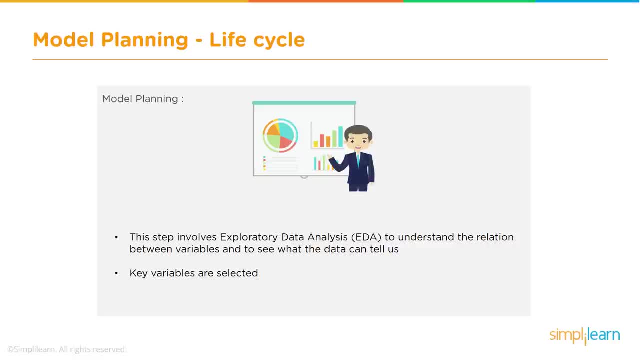 determine what kind of model you will use. you have to perform some exploratory data analysis to understand the relationship between the various variables and see if the data is appropriate, and so on. right, so that is the additional preparatory step that needs to be done. so a little bit of. 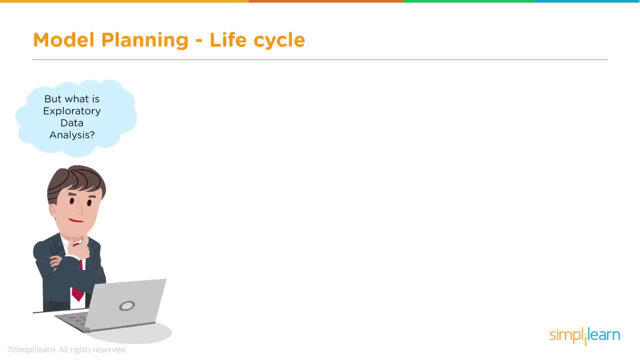 details about exploratory data analysis. so what exactly is exploratory data? analysis is basically to, as the name suggests, you're just exploring. you just receive the data and you're trying to explore and find out what are the data types and what is the. is the data clean in in each of the columns? 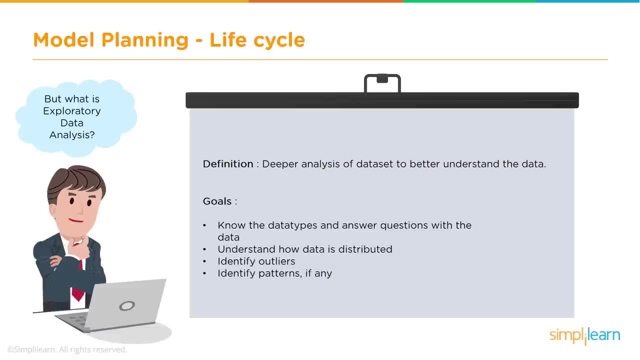 what is the maximum minimum value. so, for example, there are out of the box functionality available in tools like r. if you just ask for a summary of the table, it will tell you. for each column, it will give some details as to what is the mean value, what is the maximum value, and so on and so forth. 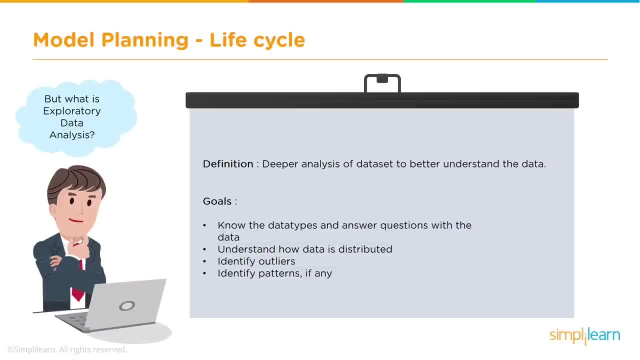 so this exercise, or this exploratory analysis, is to get an understanding of your data and then you can take steps to. during this process, you find there are a lot of missing values. you need to take steps to fix those. you will also get an idea about what kind of model to be used, and so on and so forth. 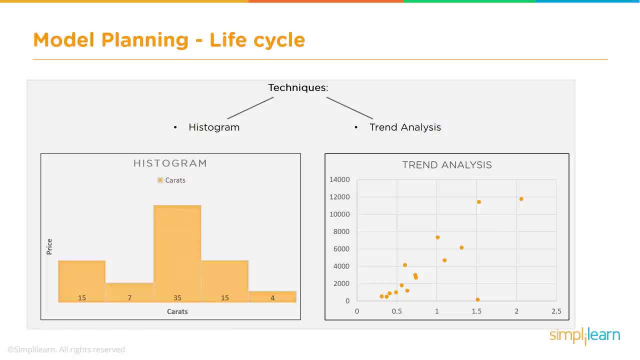 what are the various techniques used for exploratory data analysis? typically, these would be visualization techniques. like you use histograms, you can use box plots, you can use scatter plots, so these are specific ways of identifying the patterns or a few of the trends of the data, and so on. 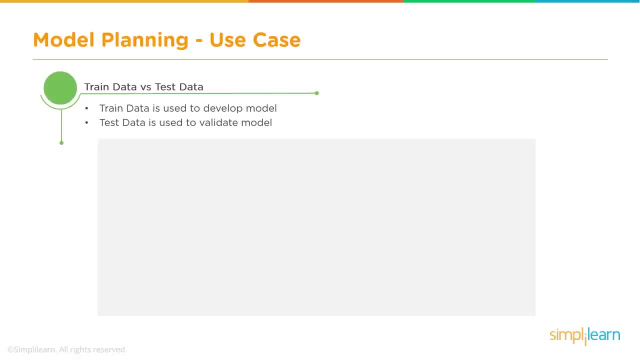 and then, once your data is ready, you you've decided on the model, what kind of model, what kind of algorithm you're going to use. if you're trying to do machine learning, you need to pass your 80% the training data, or rather, you use the training data to train your model and the training process. 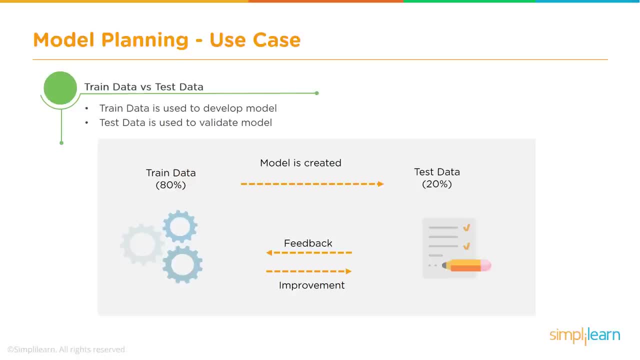 itself is iterative, so the training process you may have to perform multiple times. once the training is done and you feel it is giving good accuracy, then you move on to test. so you take the remaining 20% of the data. remember, we split the data into training and test. so the 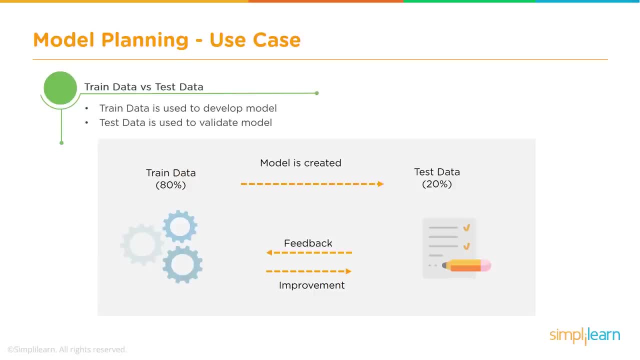 test data is now used to check the accuracy or how well our model is performing, and if there are further issues. let's say, model is still during testing. if the accuracy is not good, then you may want to retrain your model or use a different model. So this whole thing again can be iterated. but if the test process is passed, 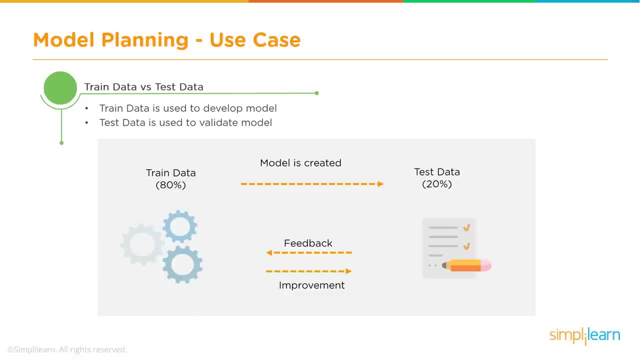 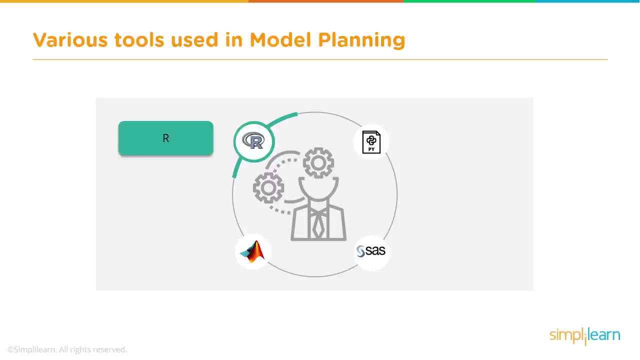 or if the model passes the test, then it can go into production and it will be deployed. All right. so what are the various tools that we use for model planning? R is an excellent tool in a lot of ways, whether you're doing regular statistical analysis or machine learning or any of these. 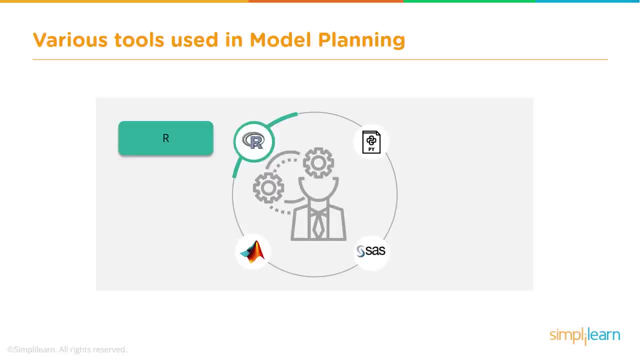 activities. R, along with RStudio, provides a very powerful environment to do data analysis, including visualization. It has a very good integrated visualization or plot mechanism which can be used for doing exploratory data analysis and then later on to do analysis, detailed analysis and machine learning and so on and so forth. Then, of course, you can write Python. 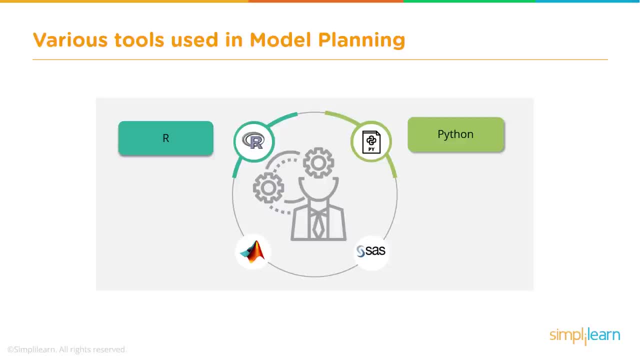 programs. Python offers a rich library for performing data analysis and machine learning, and so on, so on. MATLAB is a very popular tool as well, especially during education, So this is a very easy to learn tool. So MATLAB is another tool that can be used. And then, last but not least, 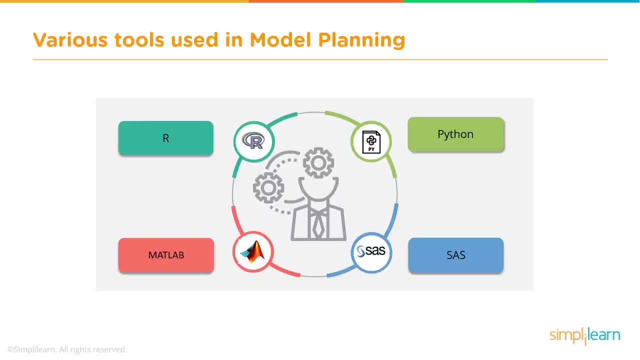 SAS. SAS is again very powerful. It is a proprietary tool and it has all the components that are required to perform very good statistical analysis or perform data science. So those are the various tools that will be required for, or that can be used for, model building, And so the 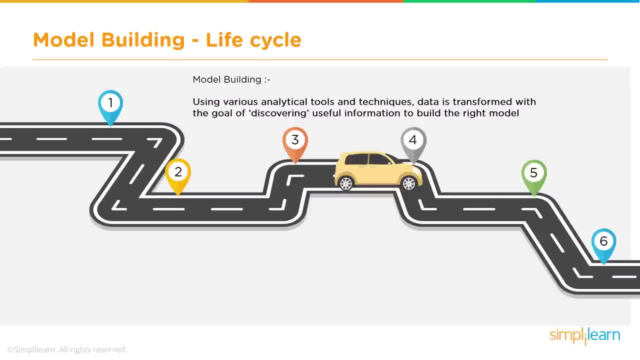 next step is model building. So we have done the planning part. We said, okay, what is the algorithm we are going to use, What kind of model we are going to use? Now we need to actually train this model, or build the model, rather, so that it can then be deployed. So what are the various ways? 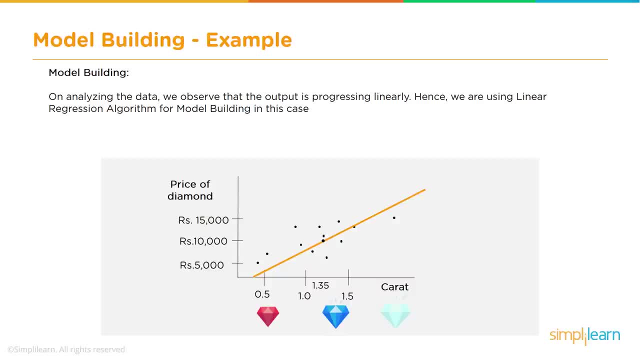 or what are the various types of model building activities. So it could be, let's say, in this particular case we have a model building, So we have a model building, So we have a model building. particular example that we have taken: You want to find out the price of 1.35 carat diamond. So this: 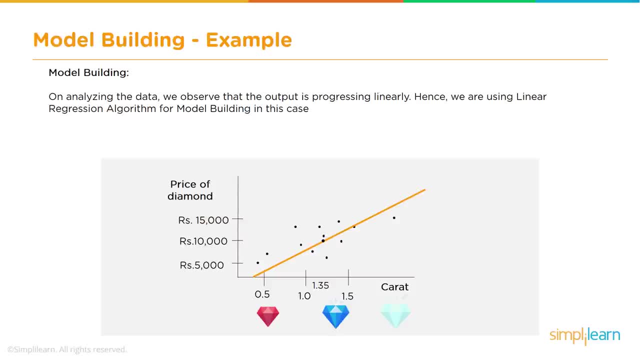 is, let's say, a linear regression problem. You have data for various carats of diamond and you use that information, You pass it through a linear regression model or you create a linear regression model which can then predict your price for 1.35 carat. So this is one example of 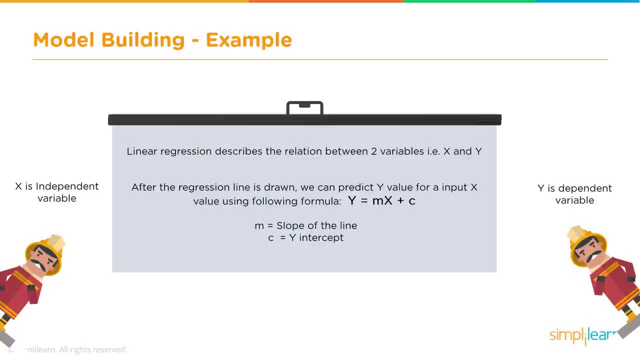 model building And then a little bit details of how linear regression works. So linear regression is basically coming up with a relation between an independent variable and a dependent variable, So it is pretty much like coming up with equation of a straight line which is the best fit for the 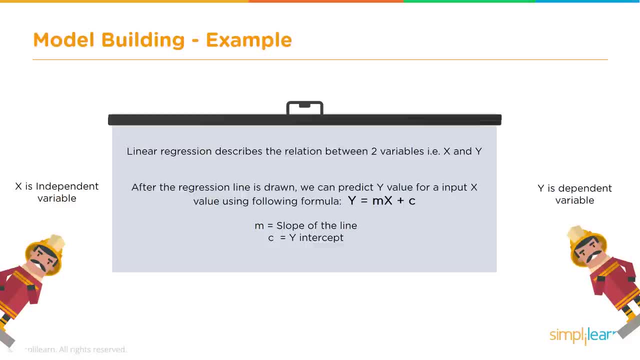 given data. So like, for example here: y is equal to mx plus c. So y is the dependent variable and x is the independent variable. We need to determine the value of the independent variable, So we need to determine the values of m and c for our given data. So that is what the training process. 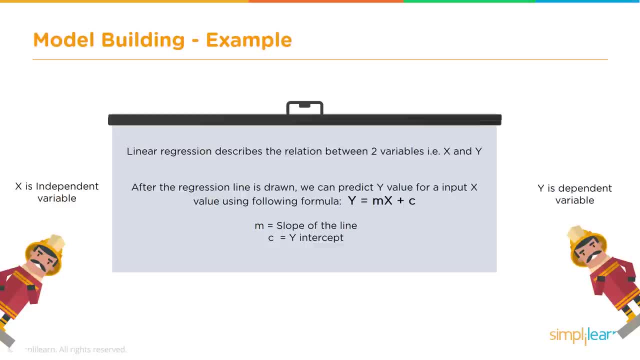 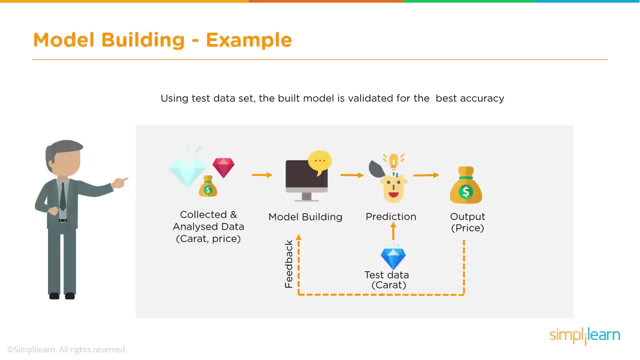 of this model does. At the end of the training process you have a certain value of m and c and that is used for predicting the values of any new data. that comes All right. so the way it works is we use the training and the test dataset to train the model and then validate whether the model 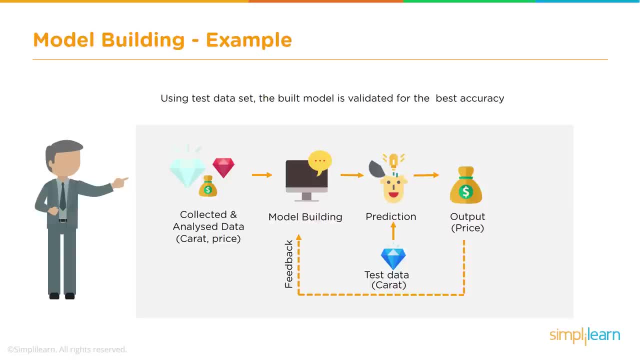 is working fine or not using test data, And if it is working fine, then it is taken to the next level, which is put in production. If not, the model has to be retrained. If the accuracy is not good enough, then the model is retrained, maybe with more data, or you come up with a. 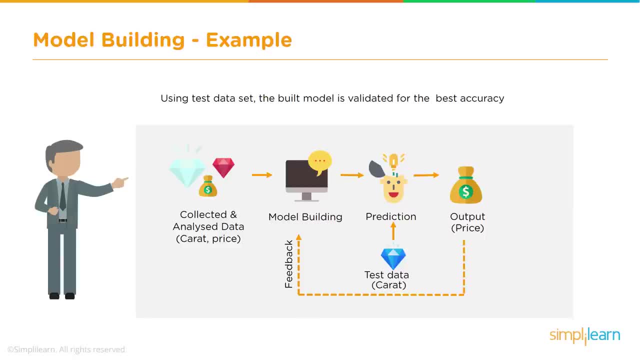 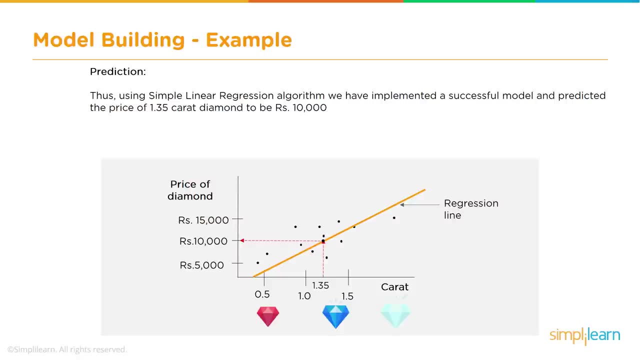 newer model or algorithm and then repeat that process. So it is an iterative process. Once the training is completed- training and test- then this model is deployed And we can use this particular model to determine what is the price of 1.35 carat diamond- Remember that was our. 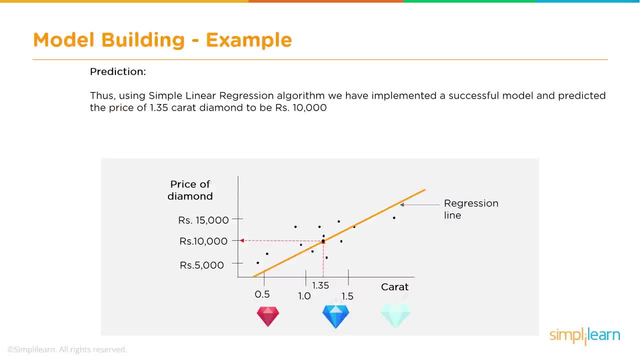 problem statement. So now that we have the best fit for this given data, we have the price of 1.35 carat diamond, which is 10,000.. So this is one example of how this whole process works. Now how do we? 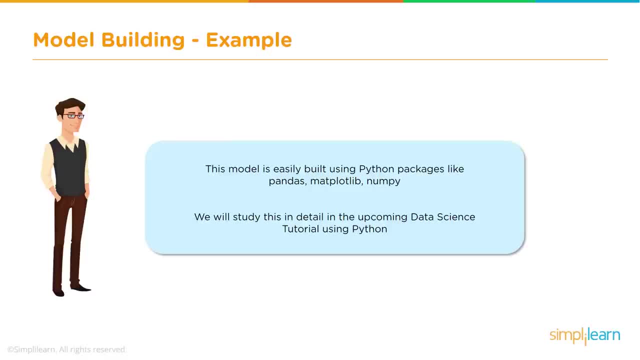 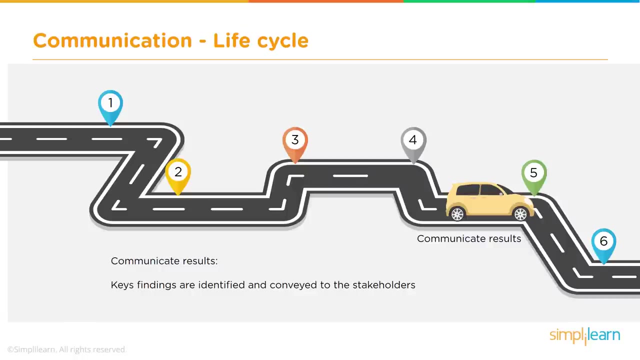 build the model. There are multiple ways. You can use Python, for example, and use libraries like Pandas or NumPy to build the model and implement it. This will be available as a separate tutorial, a separate video in this playlist. So stay tuned for that. Moving on. once we have the results, the next. 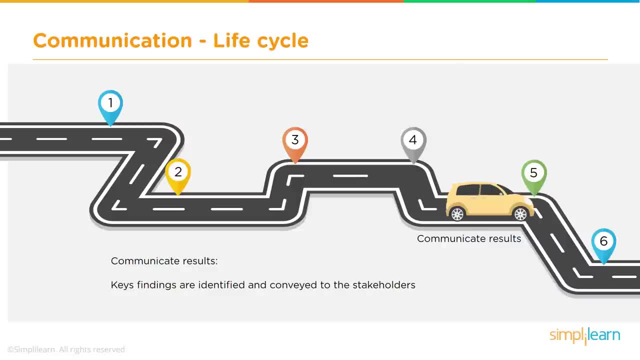 step is to communicate these results to the appropriate stakeholders. So it is basically taking these results and preparing like a presentation or a dashboard and communicating these results to the concerned people. So finishing or getting the results of the analysis is not the last step, but you need to, as a data scientist, take these. 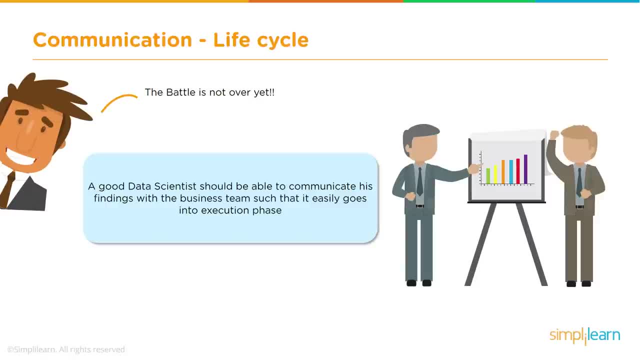 results and present it to the team that has given you this problem in the first place, and explain your findings, Explain the findings of this exercise and recommend, maybe, what steps they need to take in order to overcome this problem or solve this problem. So that's the first step. 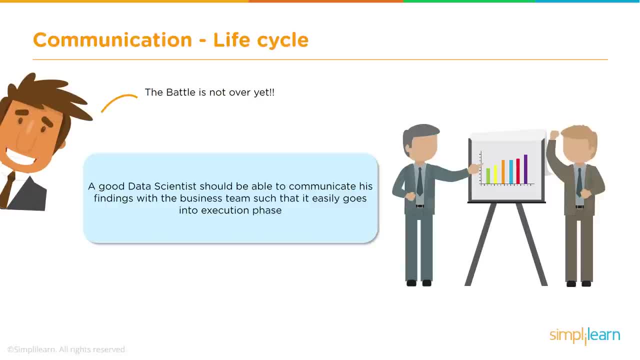 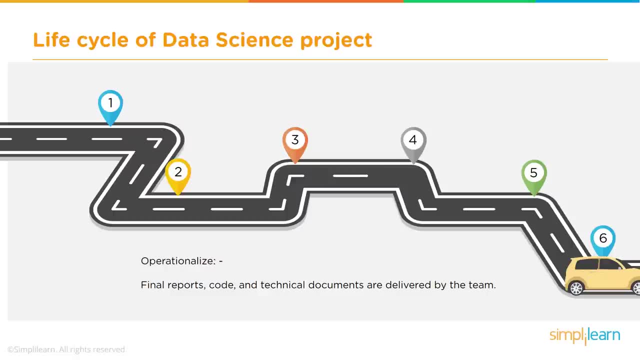 Next step is to operationalize. So if everything is fine, your data scientist's presentations are accepted, then they put it into practice and thereby they will be able to improve or solve the problem that they stated in step one. Okay, so quick summary of the lifecycle. You have a. 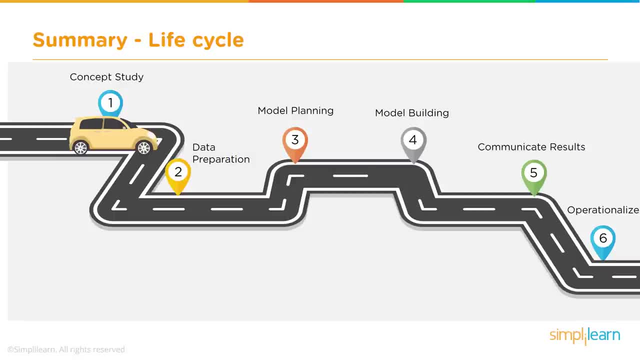 concept study, which is basically understanding the problem, asking the right questions and trying to see if there is enough data to solve this problem and then even maybe gather the data. then data preparation: the raw data needs to be manipulated, you need to do data munging so that 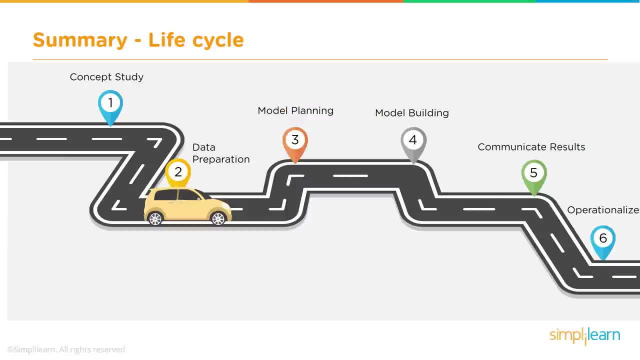 you have the data in a certain proper format to be used by the model or our analytics system, and then you need to do the model planning- what kind of a model, what algorithm you will use for a given problem- and then the model building, so the exact execution of that model happens in step four. 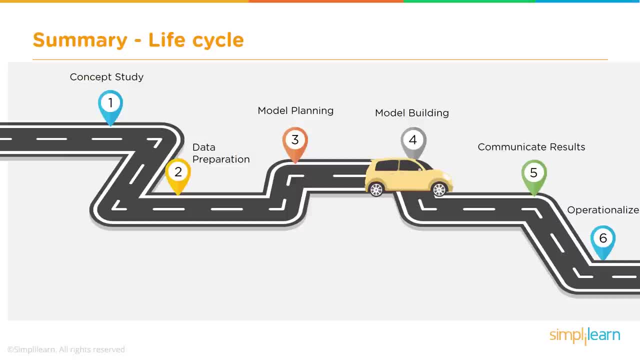 and you implement and execute that model and put the data through the analysis in this step and then you get the results. these results are then communicated, packaged and presented and communicated to the stakeholders and once that is accepted, that is operationalized. so that is the final step. now in the end, let's take a quick look at. 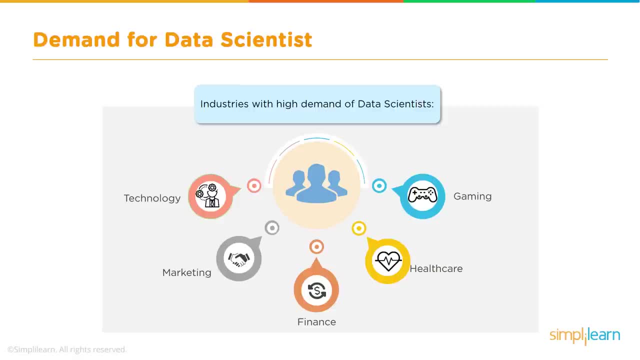 the demand for data scientists. data science is an area of great demand. the demand for data scientists is currently huge and the supply is very low, so there is a huge gap. so what are some of the industries with high demand for data scientists? i think gaming is definitely one area. 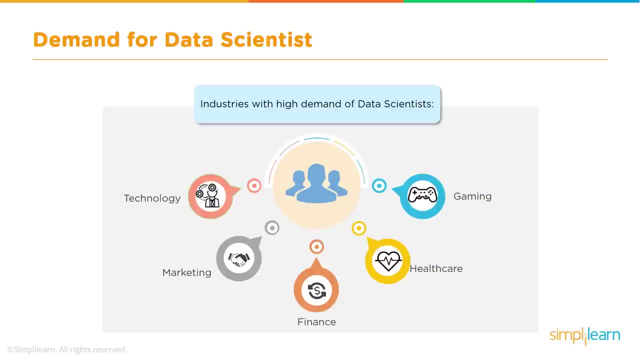 where it's a industry which is consumer-facing industry and a lot of people play games- and growing industry and it requires a lot of data science. so that's is an area where data scientists are in demand. Then we have healthcare, For example- data science. 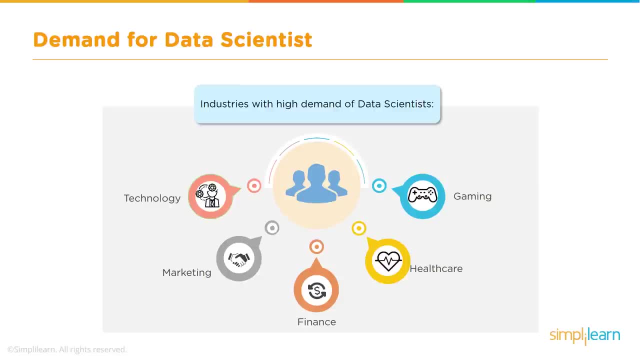 is used for diagnosis and several other activities within healthcare, predicting, for example, a disease. So healthcare is definitely finance, definitely banks, insurance companies, all of these. There is a huge demand for data scientists. Marketing is like a horizontal functionality across all industries. There's a demand for data scientists there. Then, of course, in technology, 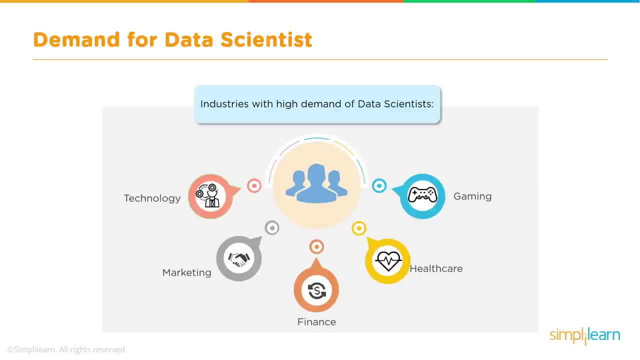 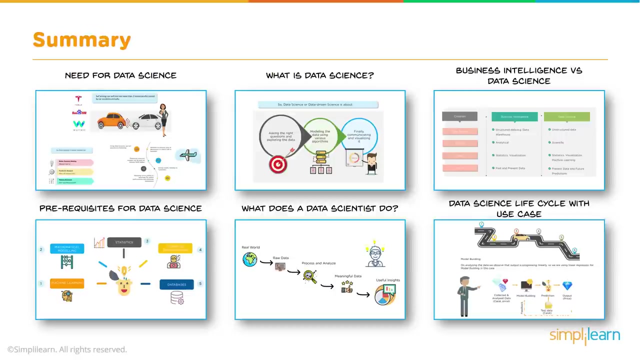 areas- So pretty much all of these areas- there is a lot of demand. Globally, there is a huge demand, So this is a very, very critical skill that would be required currently as well as in the future. So let's summarize what we have seen so far. We talked about the need for data science. 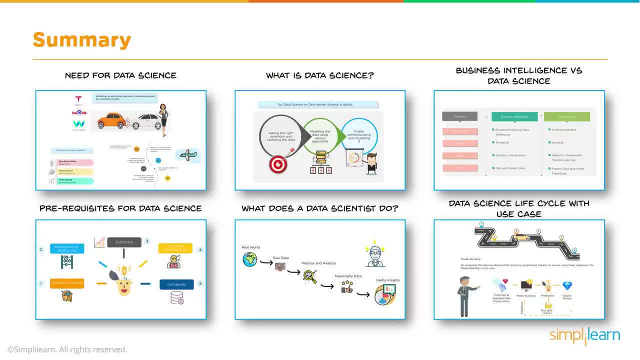 what data science can do and what is data science and what are the prerequisites of data science in terms of the skills and programming, languages and tools, And so on and so forth. We also talked about the various tools that are available, like Python and R, and we did a comparison also between business intelligence and data science. 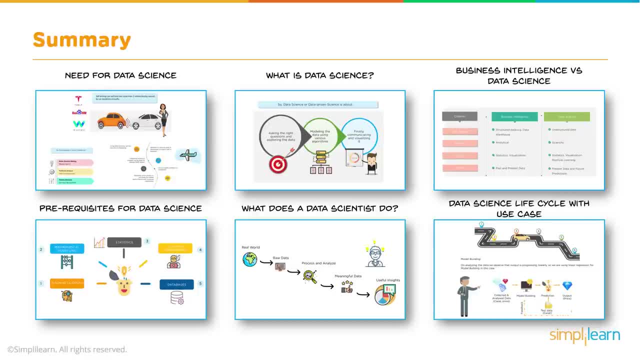 And we did a detailed discussion about the life cycle of a data science project with an example. And, last but not least, we talked about the demand for data scientists, the global demand. There's a huge demand for data scientists. We talked about that as well. 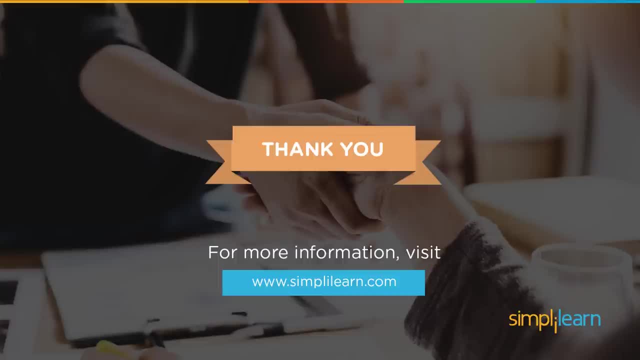 So with that, we come to the end of this session. Thank you very much. Thank you very much for watching this video, And if there are any feedback, any comments, please, or any questions, please put it below and we will get back to you. 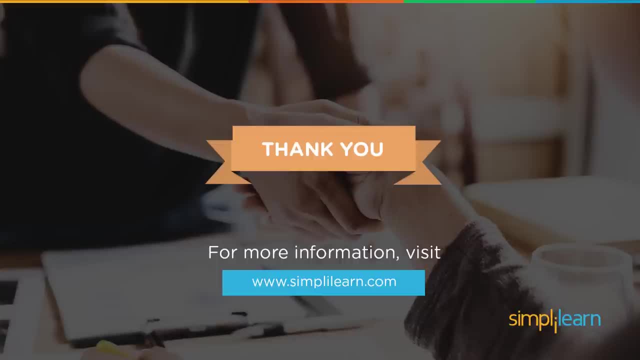 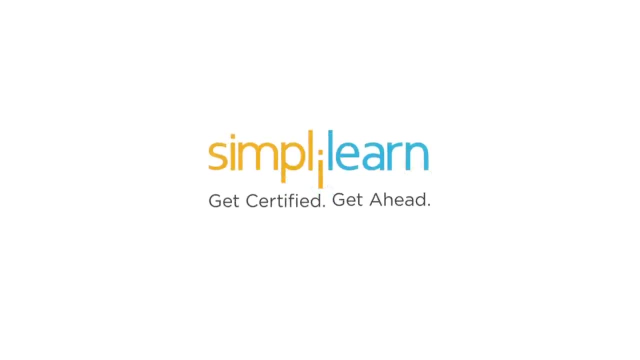 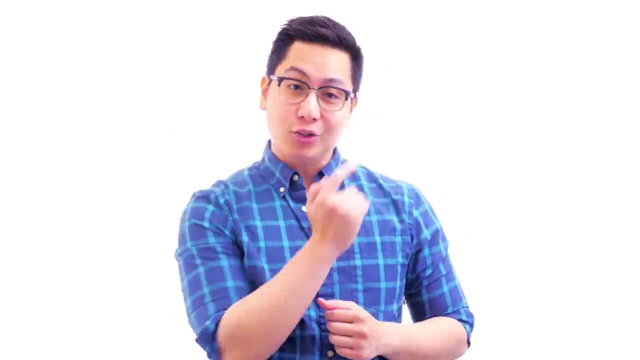 provide your contact information or email so that we can respond to you, And thank you very much once again and have a good day. Bye, bye, Hi there. If you like this video, subscribe to the Simply Learn YouTube channel and click here to watch similar videos. up and get certified: click here.